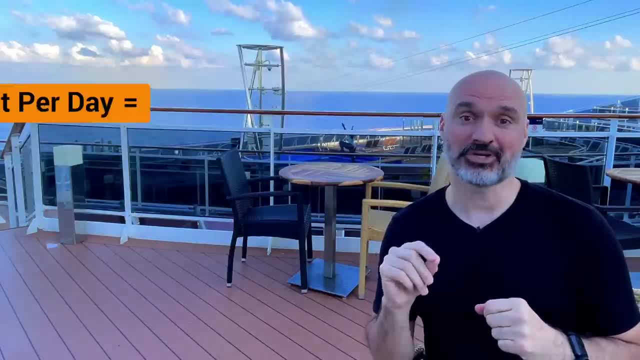 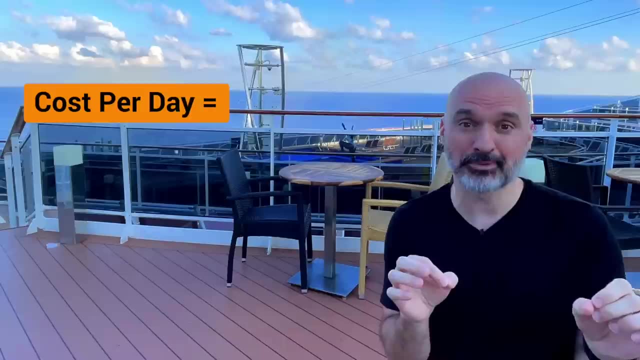 Okay, so the next term I want to talk about is total cost of a cruise. So total cost of a cruise we're going to talk about is cost per day. I don't hear a lot of cruisers talking about this number, but to me this number is the best way to compare apples to apples, cruises to cruises. 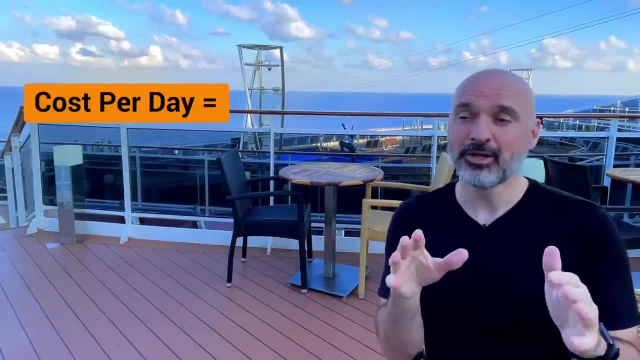 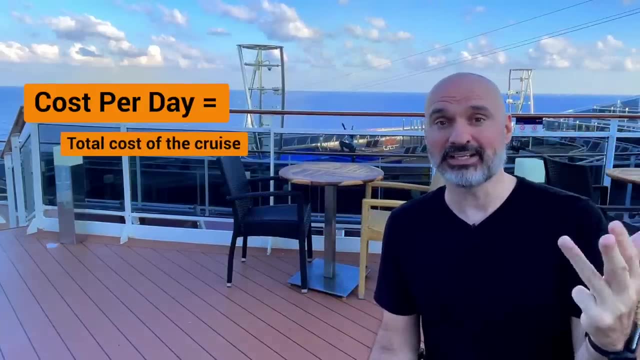 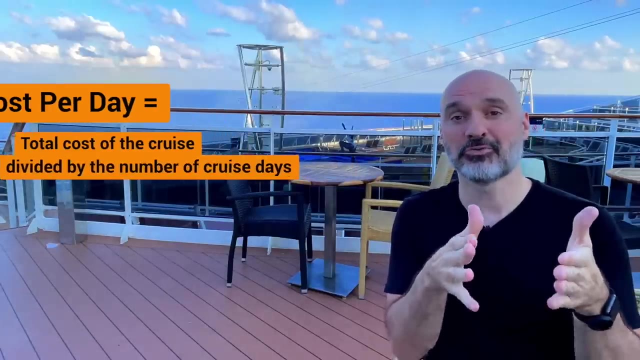 And we'll talk about cost per day more a little bit later. but that's the total cost of the cruise, which is the cruise fare, taxes, port fees and gratuities divided by the number of days in the cruise, And that'll get you what that'll give you, what that cruise cost you per day. 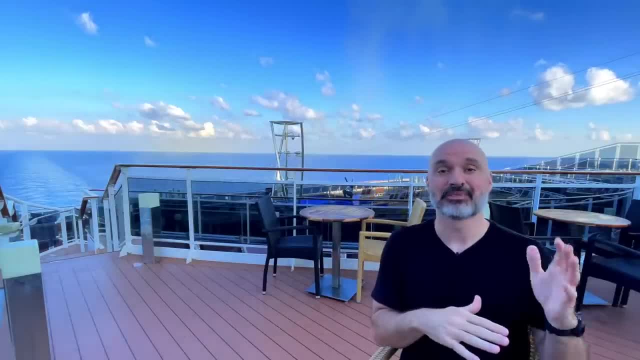 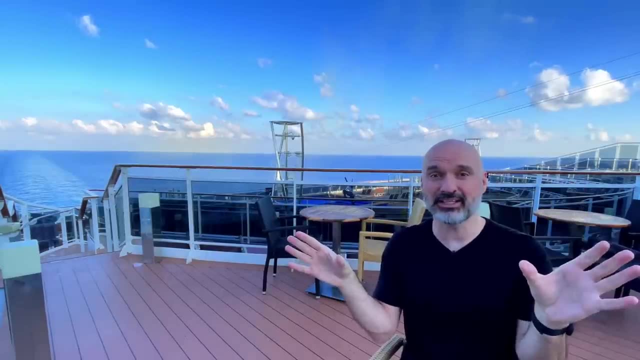 Okay, The next two terms we're going to talk about. I'm going to put them together: double occupancy and solo supplement. The reason I'm putting them together is because sometimes they're used interchangeably. They mean a little bit different thing, but they're very similar. 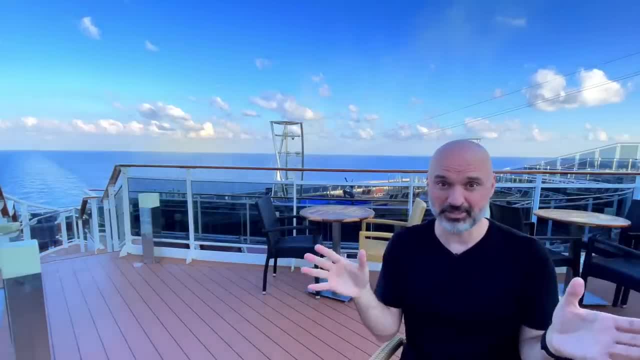 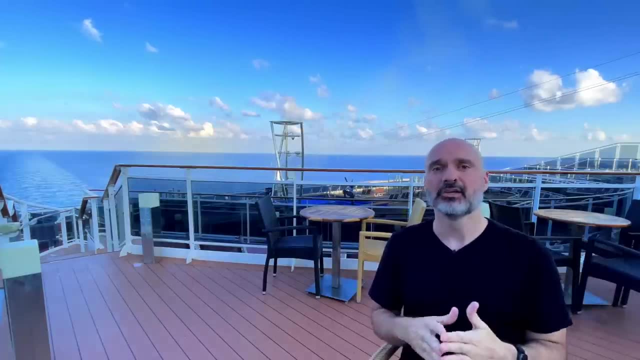 So I want to make sure you understand the difference, but also how they're used interchangeably. So a lot of cruisers talk about solo cruisers, talk about having to pay double occupancy. What does that mean? So if you go book a cruise, they'll show you a cost. Let's say it's $500 a person. 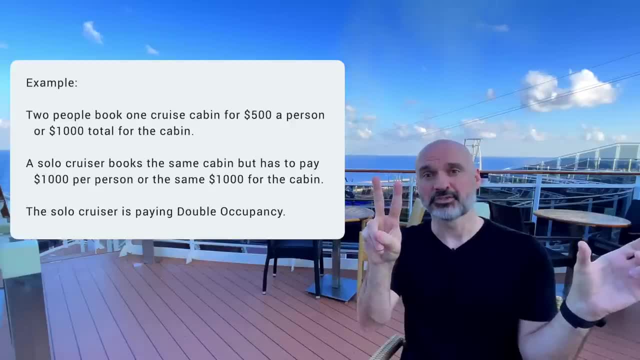 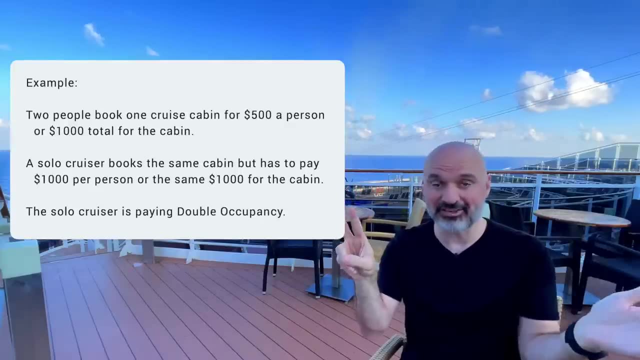 That's the price you would pay if you book for two people. So each person would pay $500.. So that cabin would cost those two people together $500 or $1,000, $500 per person. If you book it solo and it costs you $1,000, you're basically paying the cost that two people together would have to. 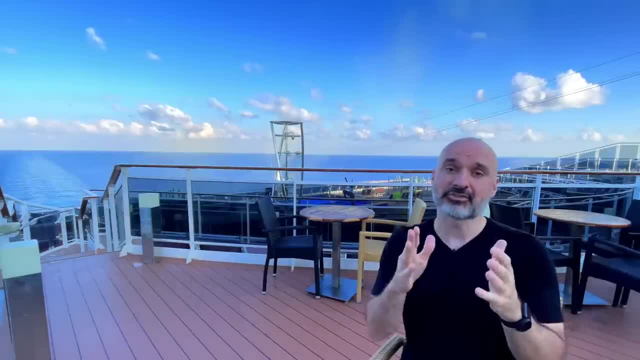 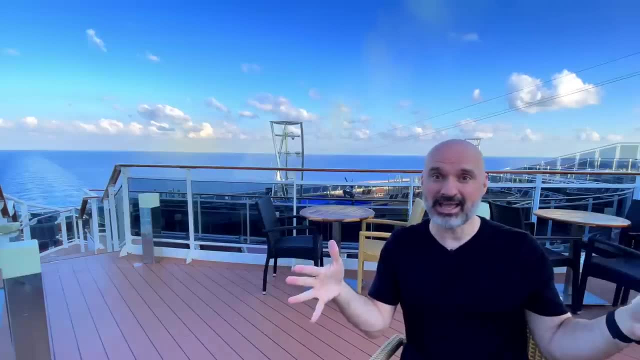 pay. So you're paying double occupancy. Now, solo supplement means how much are you paying over what an individual in a double occupancy is. So that's the price you would pay if you book for two people. So let's say someone is paying $500, like we talked about earlier- and you have to pay $1,000. 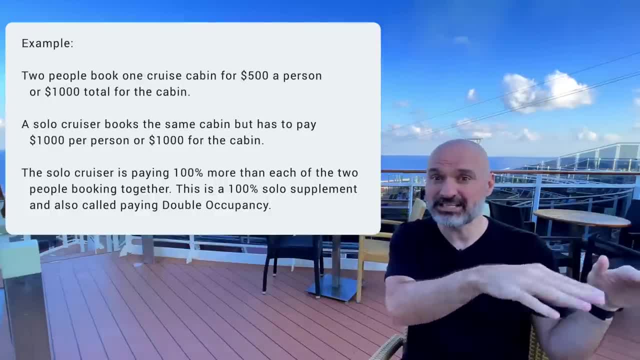 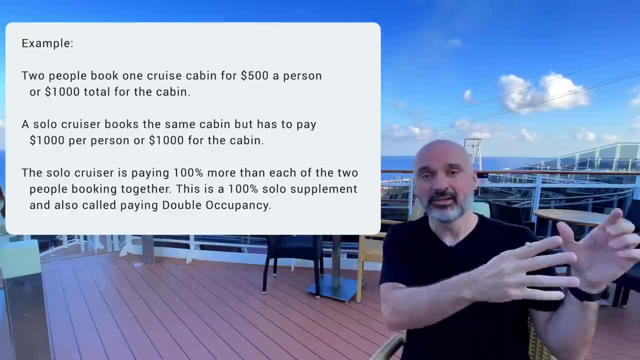 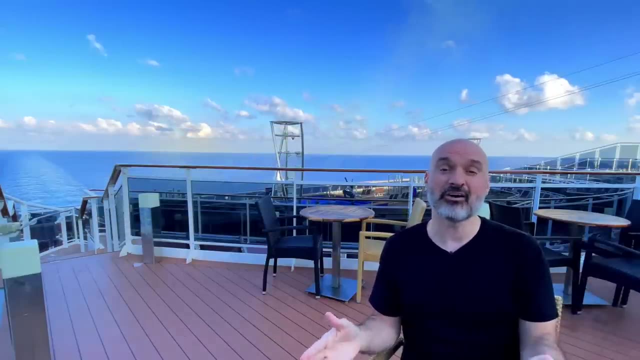 for the same cabin that two people have to pay $500 a piece for, then that would be 100% solo supplement. So you have to pay 100%. more than one person from a double occupancy cabin would have to pay. Let's say you paid $750, you'd be paying a 50% solo supplement. So the 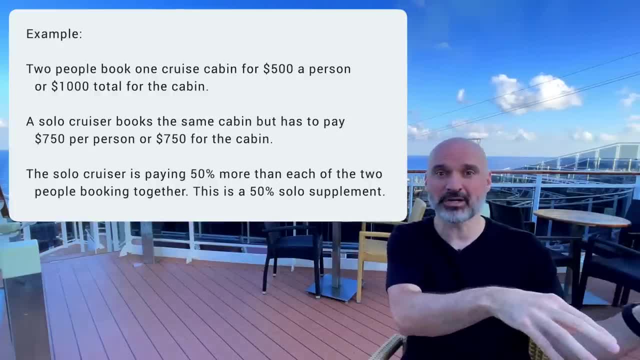 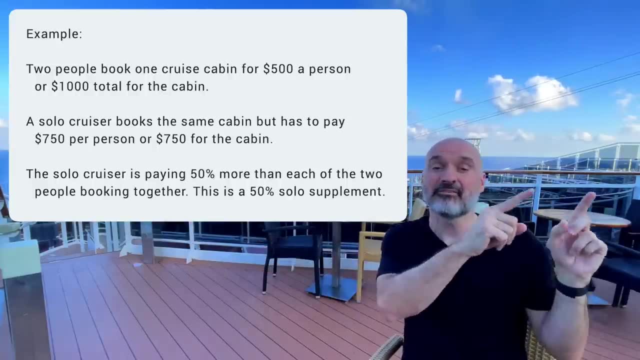 person booking a cabin with their significant other, they'd each pay $500.. So that's $1,000 they're paying for the cabin. You're paying $750 for that same cabin. So you're paying 50% more than one of those people would have to pay. So you can see how they're kind of related, but they're. 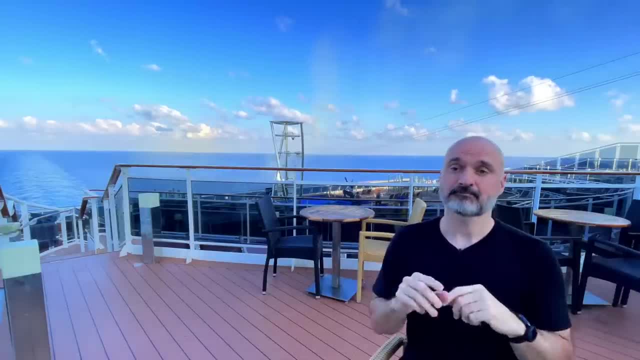 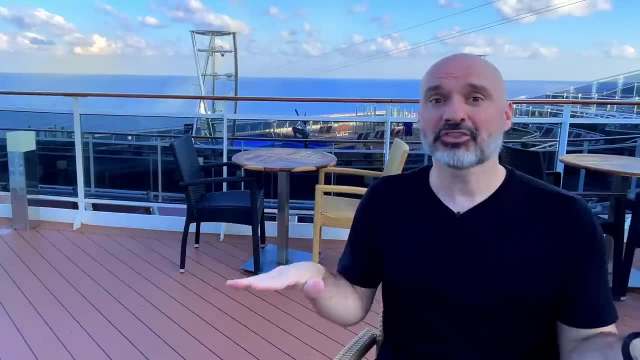 a little bit different, but I hear them used interchangeably a lot. Now I'm going to tell you something about these two terms in the cruising community. I think they're worthless. They're worthless And the number one question I get. 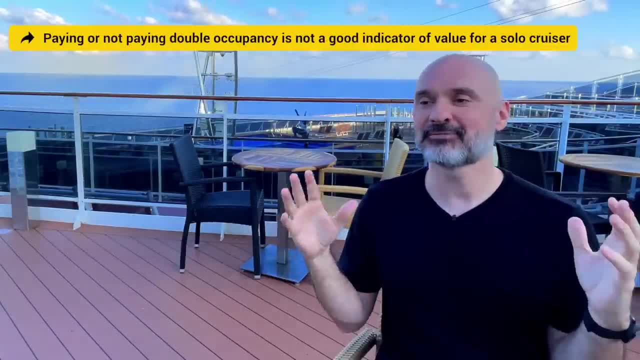 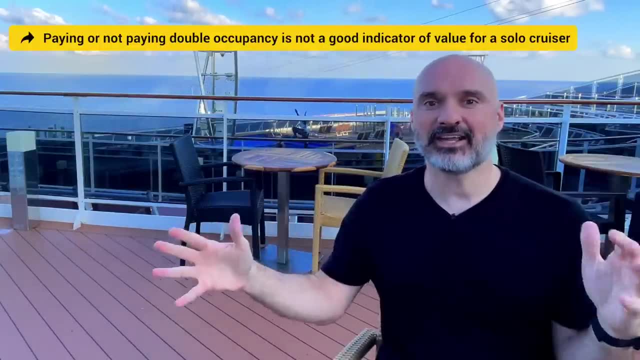 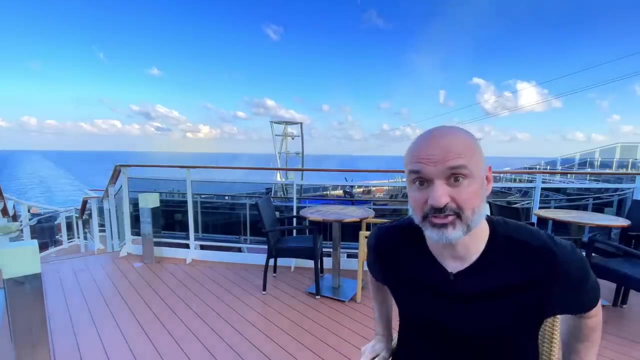 is: do you pay double occupancy? And sometimes I want to beat my head against the wall because it's such an arbitrary and worthless indicator of value for a cruise. And let me tell you why. Let me give you an example. So recently I was looking for an Alaskan cruise and I found two. 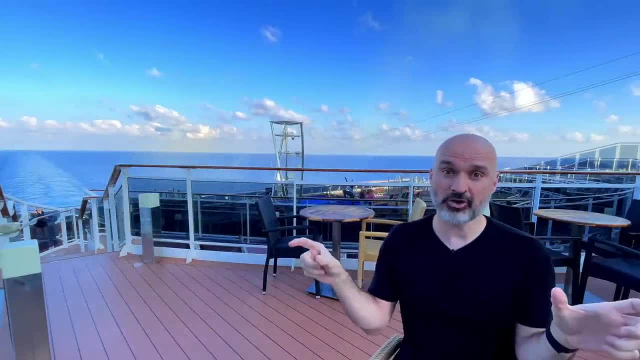 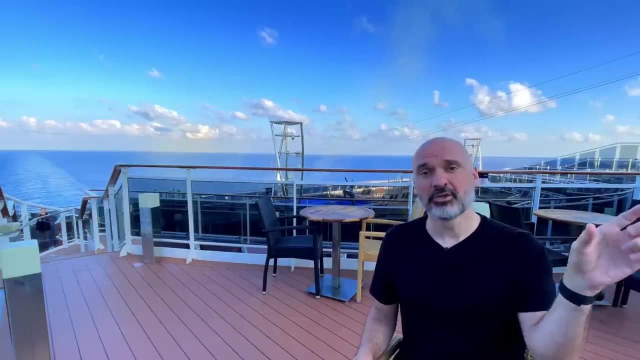 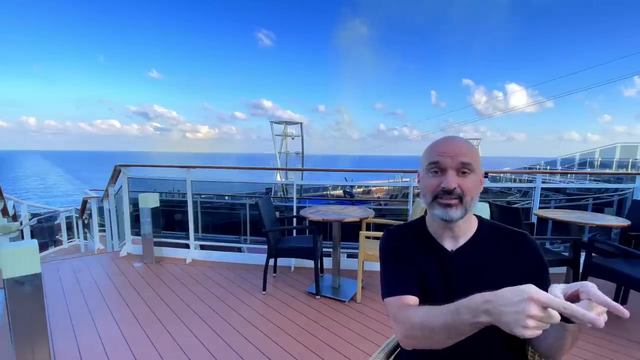 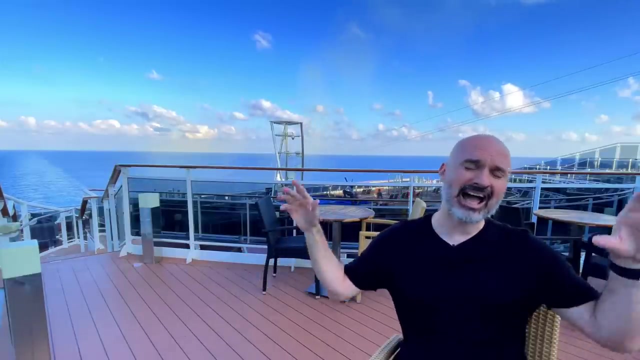 10-day cruises, exact same itinerary, one on Princess and one on Norwegian. So the Princess cruise was $450. Per person for double occupancy. So two people booked that cruise. They pay $900 for that cabin- $450 a piece. I went to book it, It was $900, double occupancy. Ah, everybody freak out. 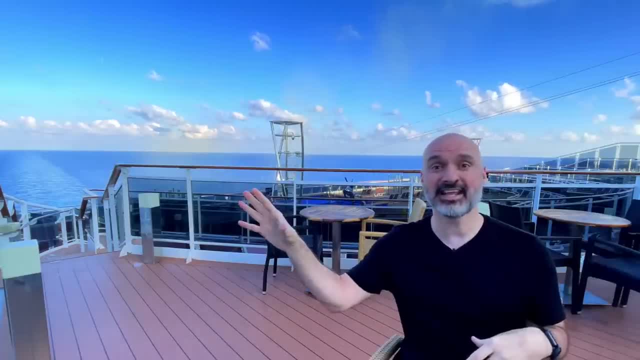 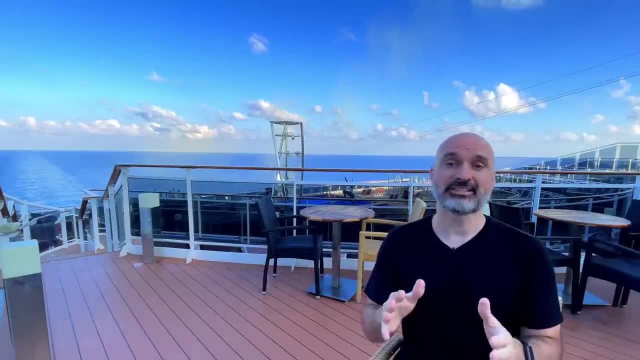 Got to pay double occupancy. all right, $900.. It's a 10-day cruise. We talked about cost per day earlier. right, It's a 10-day cruise. So it's a $90 a day cruise, all right. I looked at the. 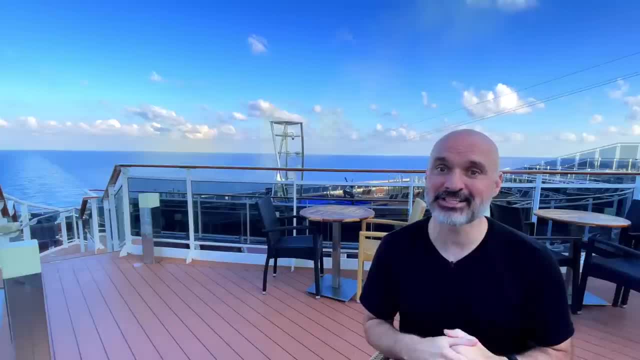 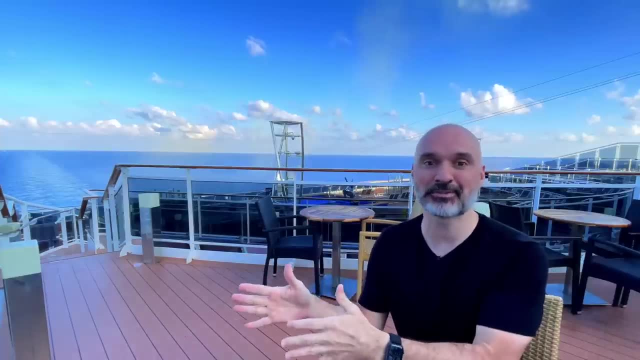 exact same cruise on Norwegian. It only had 50% solo Supplement must be a great deal compared to the Princess cruise, right? You're not paying double occupancy, You're only paying 50% solo supplement. It must be a great deal, right? Well, the cost of 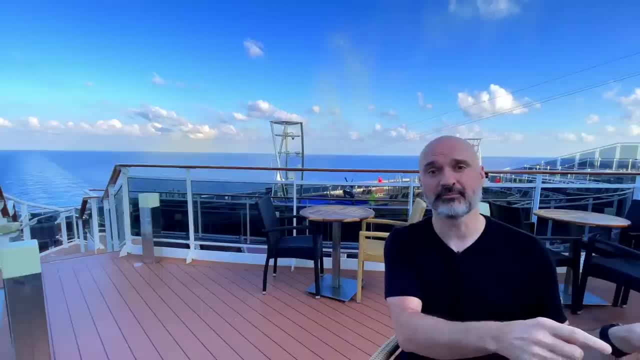 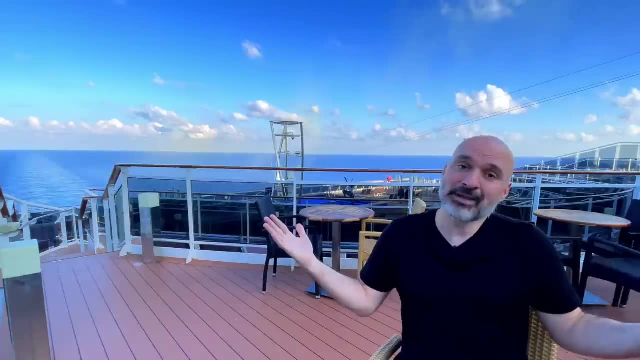 the cruise was $1,000 per person if you paid double occupancy, So it was two people booking a cabin $2,000, $1,000 a person. For me, I'm only paying 50% solo supplement, So I get that same. 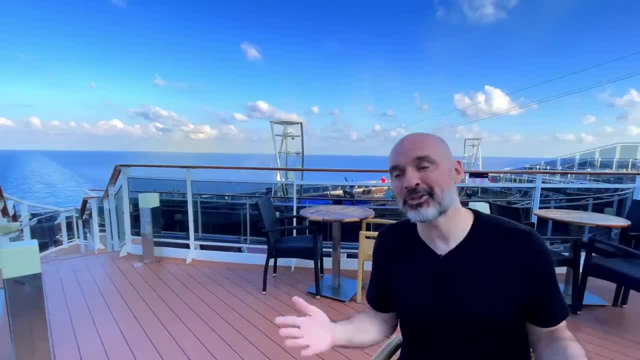 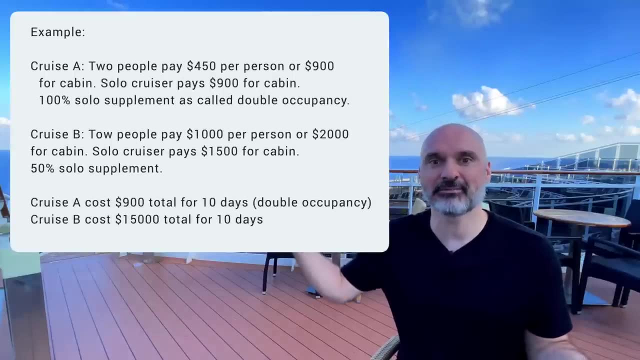 cabin for $1,500. What a bargain right, I'm only paying 50%, paying double occupancy. well, what is that? what is that, divided by 10, 1500, divided by 10, 150 a day, so i can take the exact same cruise on princess for 90 a day, paying the dreaded double occupancy? 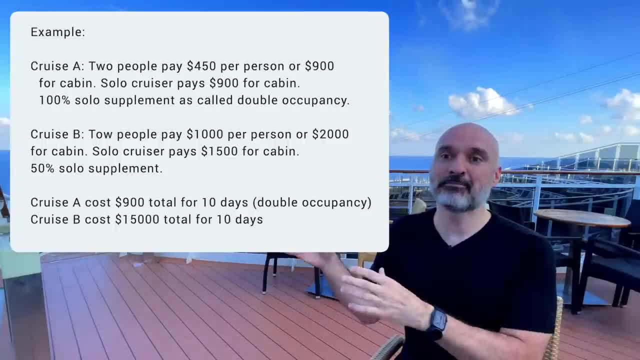 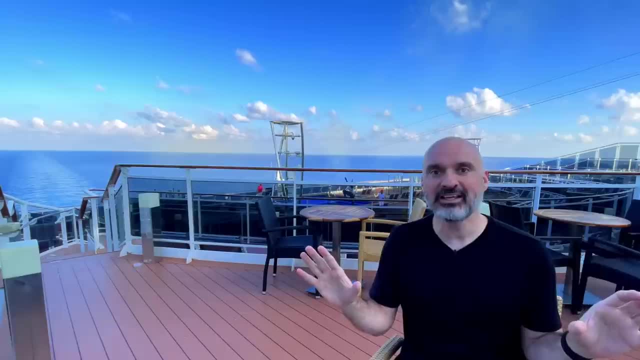 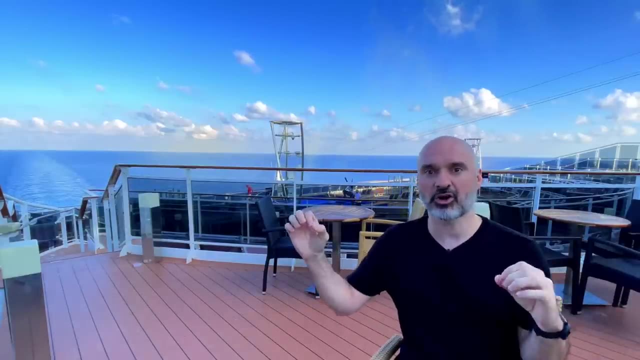 oh my god. double occupancy or i can pay half of double occupancy, getting a great deal, and pay 150 a day. so you can see why that number is arbitrary and it's not a good indicator of value. you only get an indicator, a good indicator of value, when you figure out what the cost per day is and then 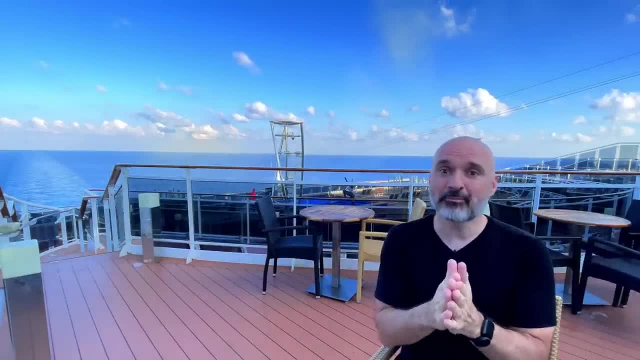 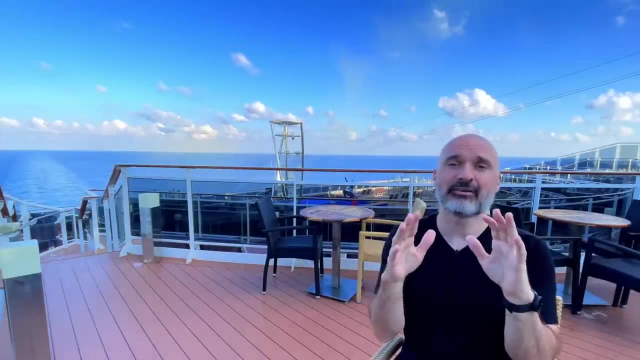 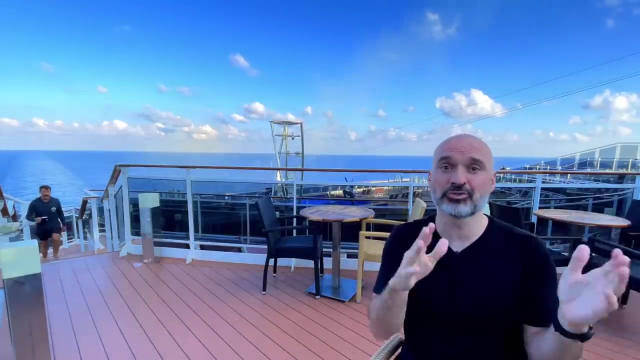 you compare apples to apples. so don't get hung up on occupancy, double occupancy, pain, double occupancy. don't get hung up on what the solo supplement is, because they really aren't an indicator of value for you as a solo travel traveler. when you compare cruise to cruise- okay, the last term i want to talk. 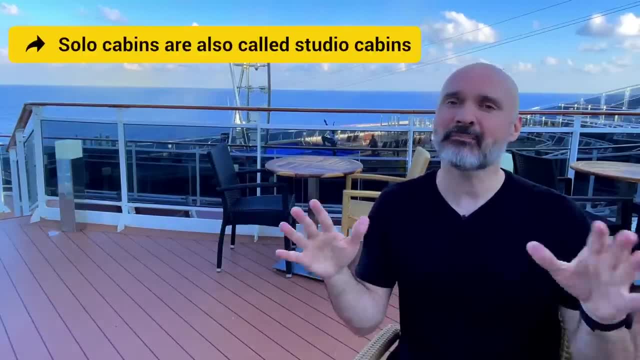 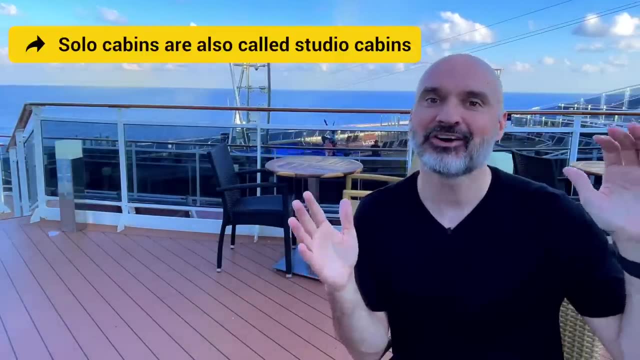 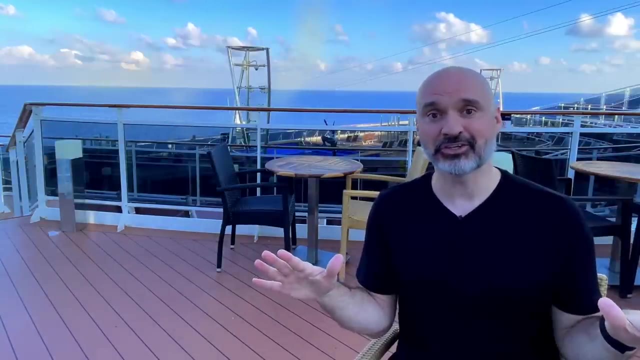 about is solo cabins, because i know if i don't mention it it'll come up. but what about solo cabins? you pay zero solo supplement. they're such a good deal. all solo travelers should travel on in solo cabins and only travel with norwegian. so in my experience, solo cabins are not a good deal. they're. 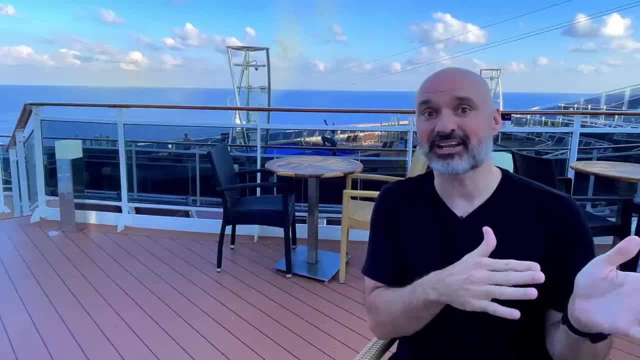 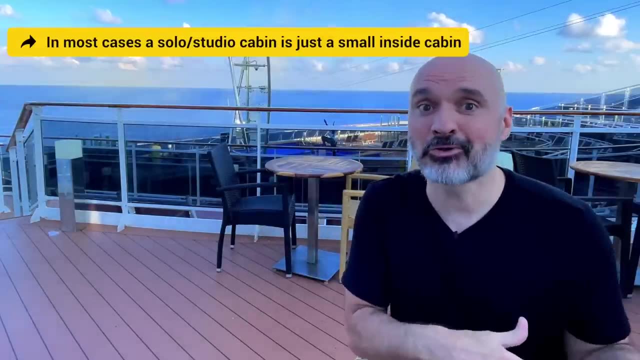 usually actually more than the inside cabin on the same exact cruise, and you know what you call a solo cabin, or you know what you call an inside cabin: that you book solo. it's a solo cabin. okay, it's actually a bigger solo cabin because solo cabins are usually much smaller than inside. 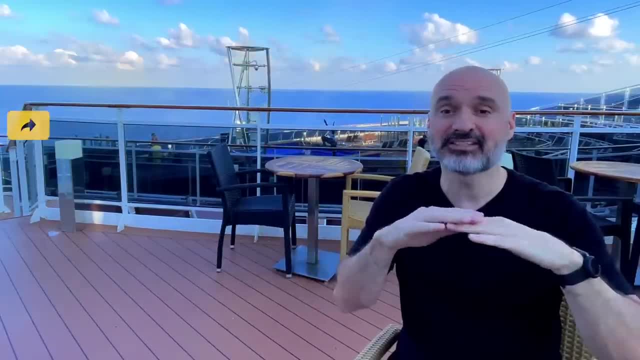 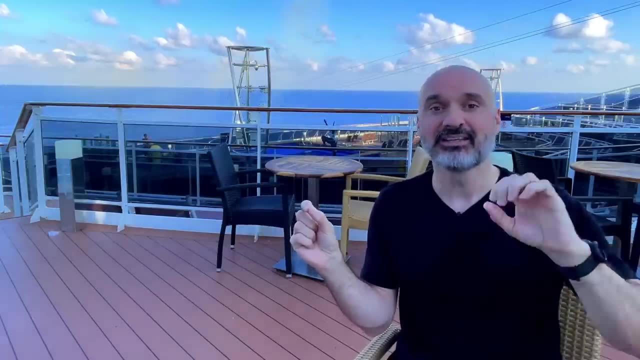 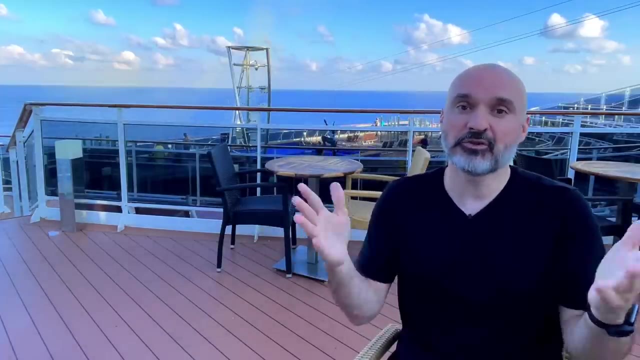 cabins and in almost every situation where i have compared prices online, the solo cabin is always more expensive than the inside cabin. and i get it. i know the norwegian people are going to jump in here and say: but you get the studio lounge well, if you, if you want to pay a premium for the studio. 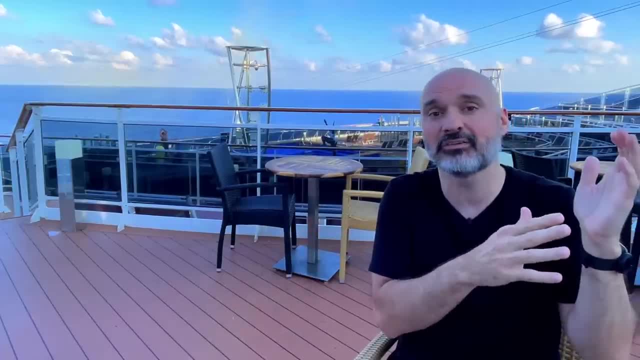 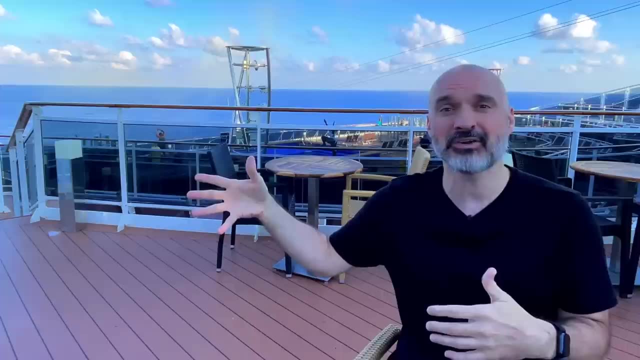 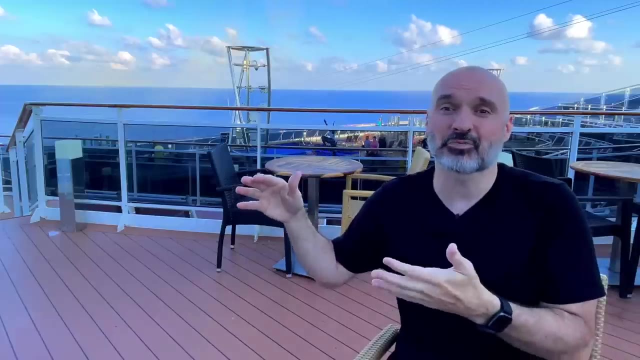 lounge you can. i'm going to be sailing on a ncl ship in a studio cabin so i get to see what all the hype is about. but if a cruise is 150 a night for the studio cabin it's going to be a lot more and 90 a night for the inside cabin on a norwegian cruise. i don't think the solo lounge is worth 60. 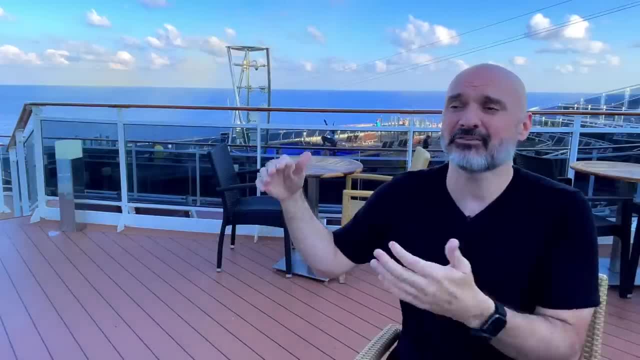 a night, which would be 600 on a 10-day cruise. i i don't think it's worth that. maybe it is to you, but it probably i'm. i'm probably going to think that it's not worth it, but we'll see. i'm going. 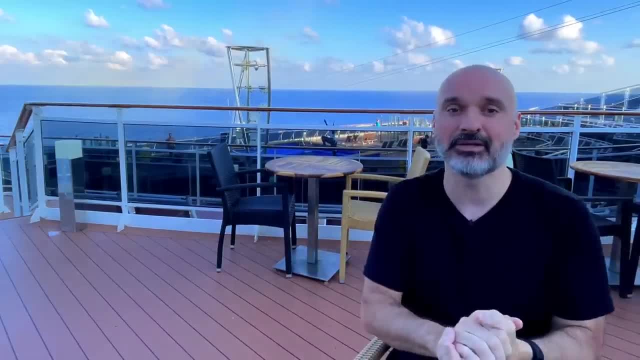 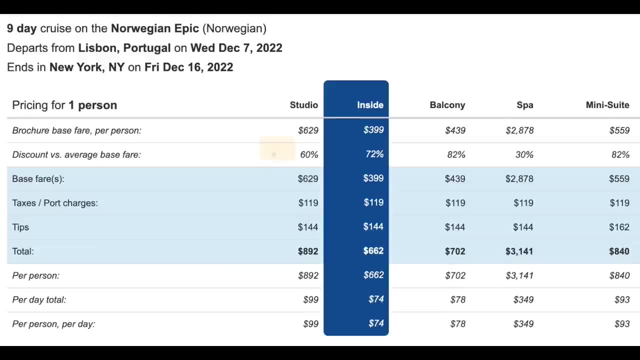 to be on ncl, uh getaway, and i'll be in a studio cabin. but yeah, i think studio cabins are kind of a marketing gimmick. and let me give you one more example. let me show you this: uh norwegian cruise here. so you'll see, here's the price of the solo cabin and the inside cabin on a norwegian cruise. 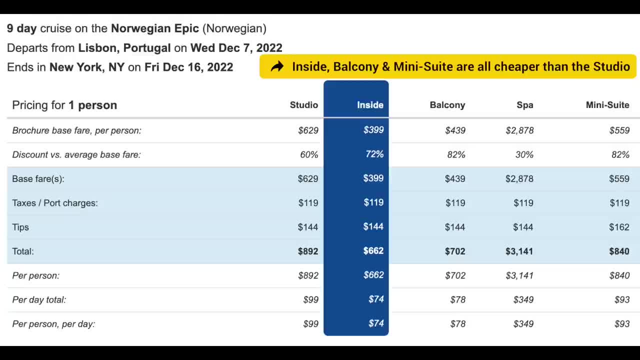 cabin, you can see that the inside cabin are both cheaper. but check this out: the mini suite was cheaper this day when i was looking at it. i don't know why. some kind of price anomaly. even though i'm paying solo supplement on the mini suite, it's still cheaper, again, solo supplement double. 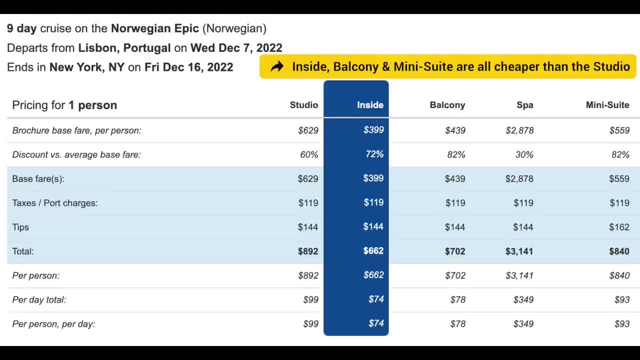 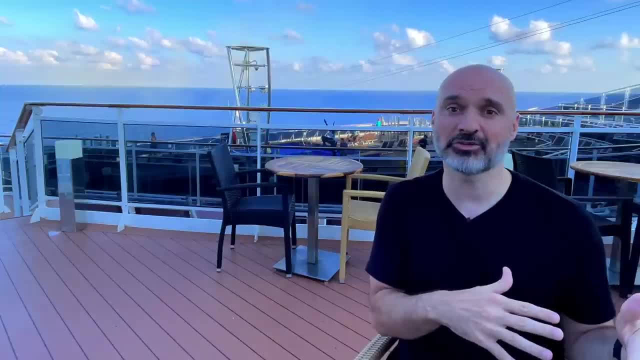 occupancy are not a good indicator of price. studio cabins: you pay no solo supplement at all, but in my experience they cost more per day than an inside cabin, usually than an ocean view, sometimes more than a balcony and an inside cabin usually more than a balcony and an inside cabin usually more. 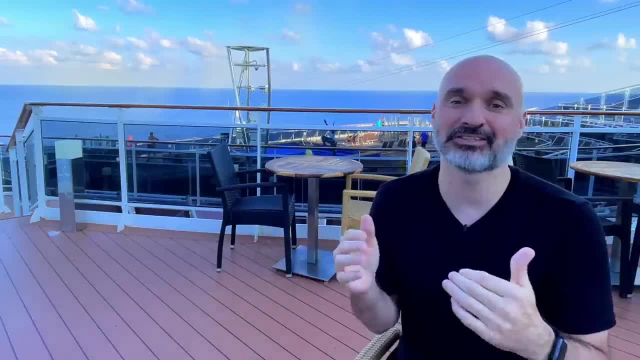 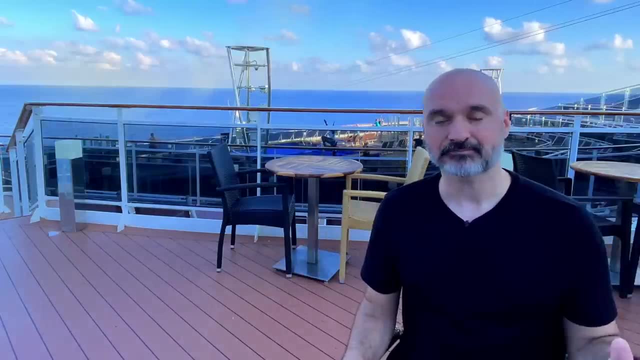 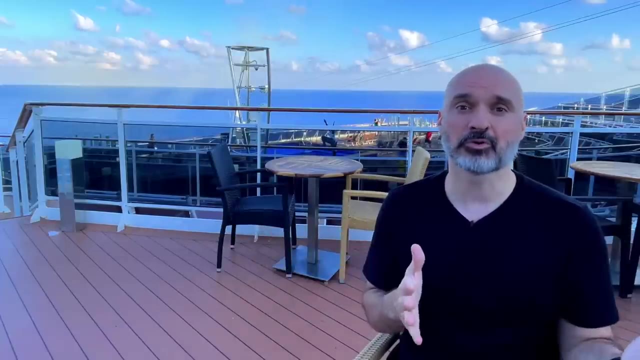 rare cases more than a mini suite. you'd be nuts to book a studio cabin over a mini suite. that's the studio cabin's more expensive. you'd be crazy. okay, enough about that. uh, we're going to jump into cruise plum here and i'm gonna show you my favorite way to find affordable cruises and 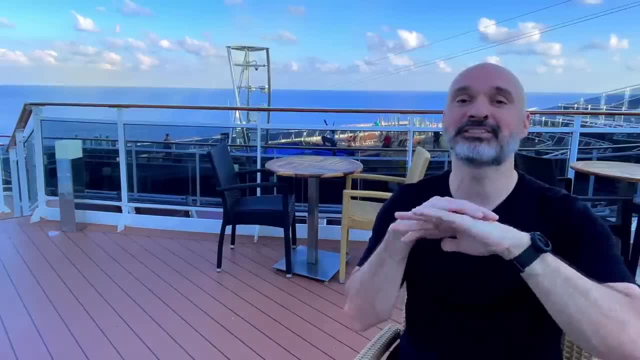 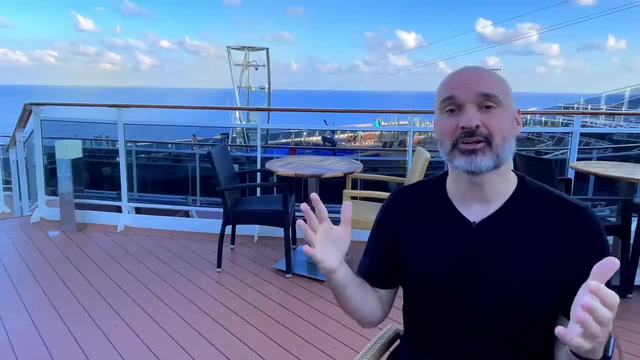 one of the great things about it is for those of you who ha, who are addicted to solo supplement amount, you can actually search by how much the solo supplement is and uh, but you can also search by how much the solo supplement is and uh, but you can also search by how much the solo supplement is. 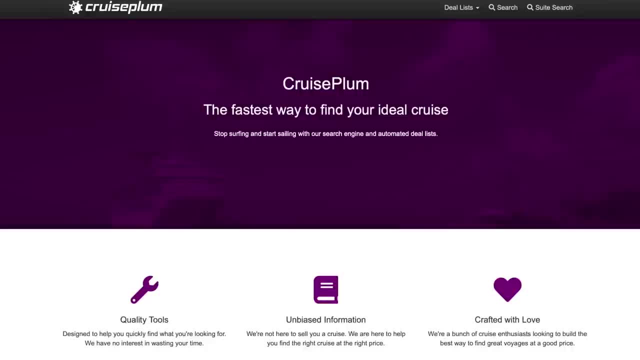 cost per night. all right, let's jump into this favorite way to search for cruises. i know a lot of people love vacations to go cruise direct and some other things, but i've found that this is the best way to search, especially as a solo cruiser. i haven't tried it as. 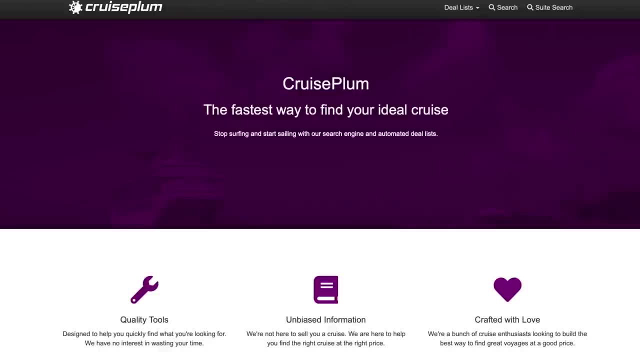 a non-solo cruiser, but it seems like it'd also be good for people searching for two, three and four person occupancy in a room or in a uh on a cruise ship. you'll see right here: it says you know. it says you know you're not allowed to book cruises with them. it's just a search engine. 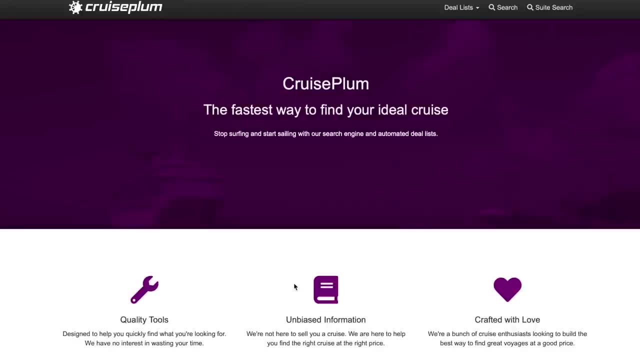 you're not allowed to book cruises with them. it's just a search engine. they're cruise enthusiasts that know how to design search engines and that's all it is. i don't know how they fund this, but there's nothing you can buy on here. you can just use it, and it's a great tool. so i'm going. 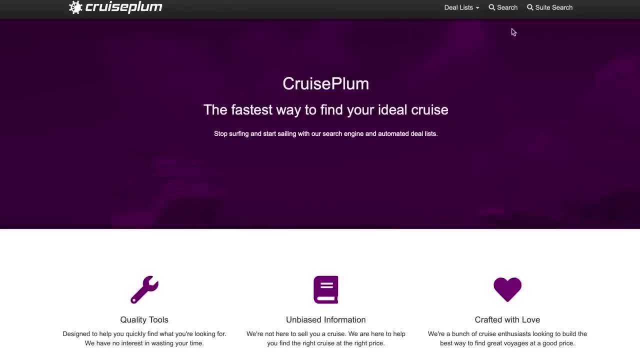 to show you a couple of ways to search on here. my favorite is just the search function, which we'll come back to in a minute, and i'll show you why it's my favorite. but if you're kind of lazy, you don't want to do a lot of work. there are some pre-made menus for you. i'll go through them. 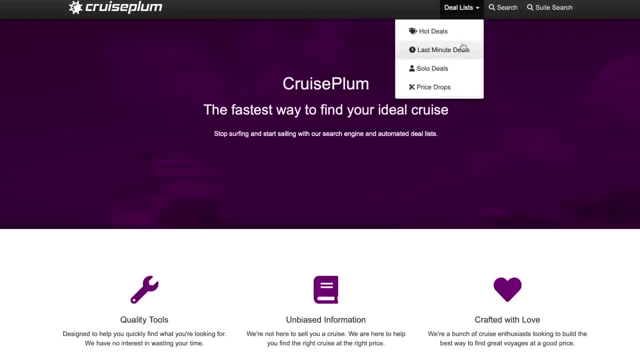 really briefly here, these three price drops, last minute deals and hot deals. they're not the greatest place to find solo deals. obviously, solo deals is probably better. search is even better than solo deals, but we'll get more into that in a minute. but i want to go over each of these real 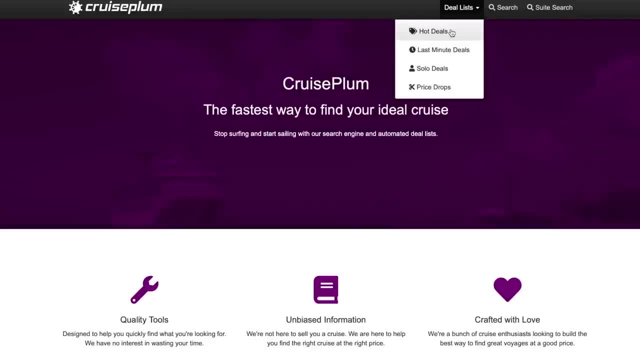 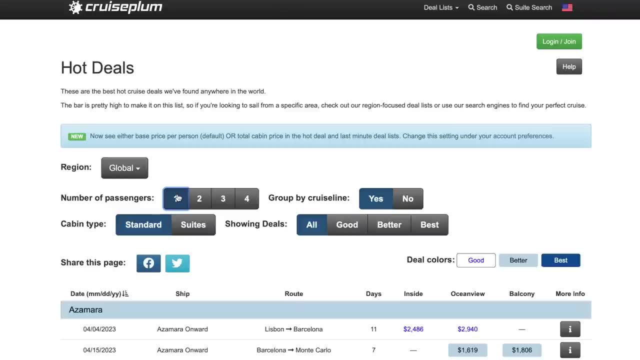 quick so you can see them and see why the functionality on this website is so good. so you click on hot deals and you can see here. you can search by number of passengers and it'll give you the price that you would pay for the cruise based on the number of passengers you select. so 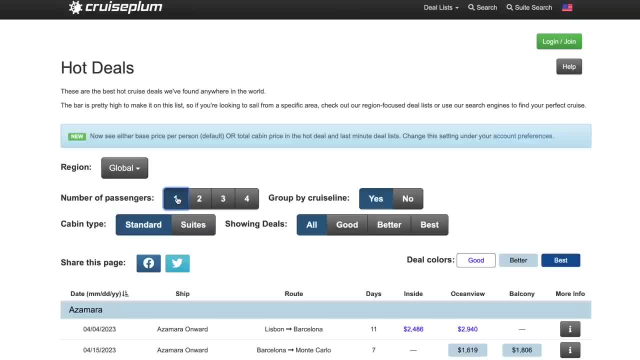 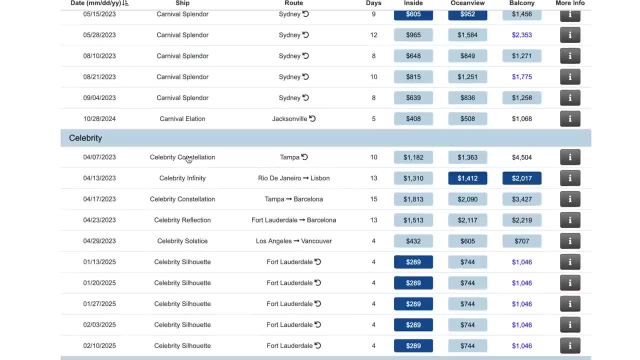 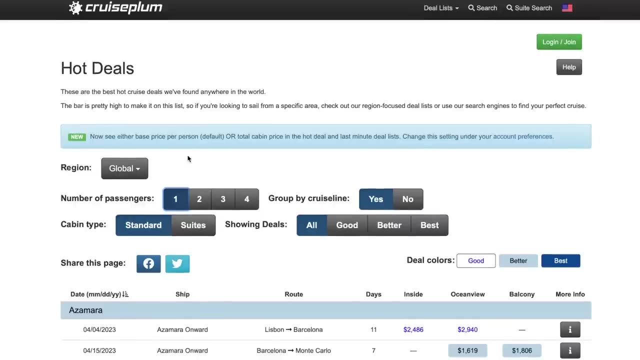 right away. it's already superior over most other ways to try to find cruises. if you're a solo cruiser, you can sort by region. so there's a ton of stuff here. you'll see. right now this is just hot deals, remember, and i don't know how they classify a hot deal. to be honest with you, i don't really. 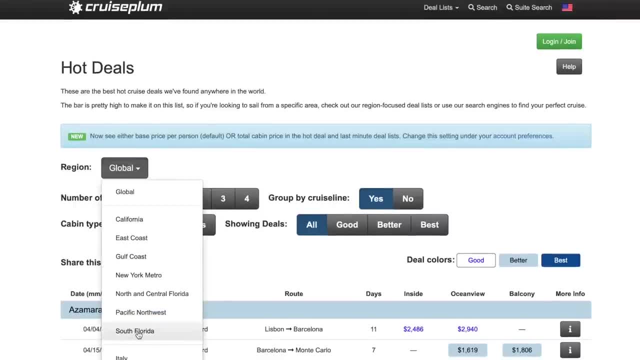 use this one very much, but it's here. but you can, you know, say you're leaving out of south florida. narrow it down, click on south florida and you'll be able to see all the hot deals in south florida. i'm on a ship right now, so my internet's not the fastest. there we go so you can see what's going. 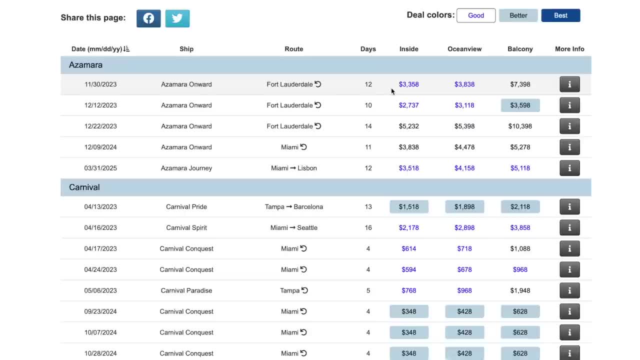 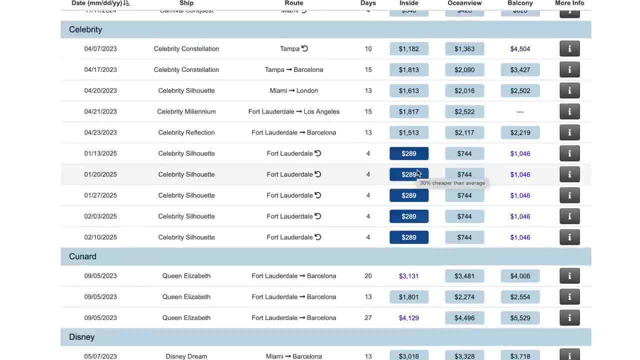 out of, you know, south florida. you got azamara, which is an expensive cruise line. everyone knows that. but you can see some deals here and the cool thing about the functionality of this website is you can go ahead and click on the cruise you're interested in. so let's say you want to go on. 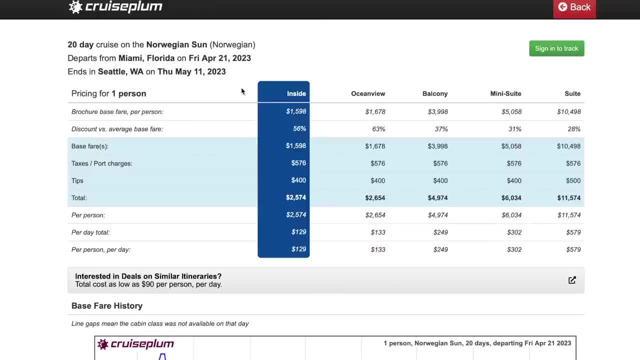 norwegian sun. i almost took this cruise, by the way. i love data and this gives you all kinds of great data that you can make an educated decision on what a cruise is going to cost you. so you'll see- it has the base fare here- what the taxes are, what the tips are. 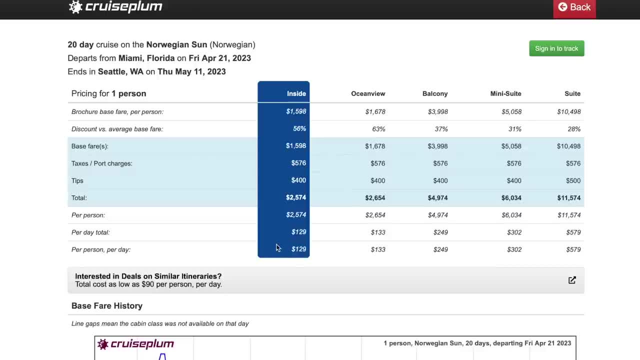 and the total cost, and it gives you the cost per day, which is my favorite metric, and then you can see what the other cabins cost. sometimes you'll see other cabins are cheaper than the inside cabin. in this case, the ocean view is only four dollars a day more. 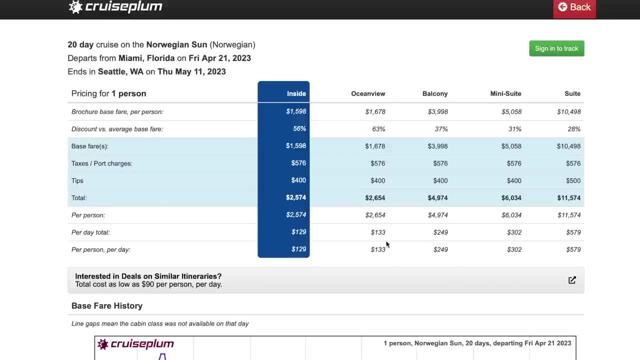 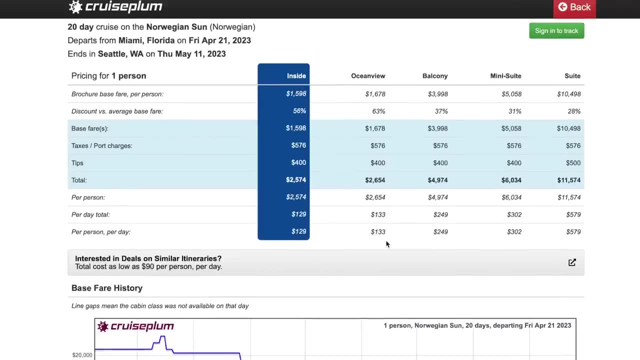 on this cruise, which i believe is 20 days, would be, you know, about uh 80 dollars more so not to you know, not too much more expensive, uh for this cruise. i think this is an alaskan cruise as well, or no? no, this is a panama canal cruise, i think so it'd be probably. 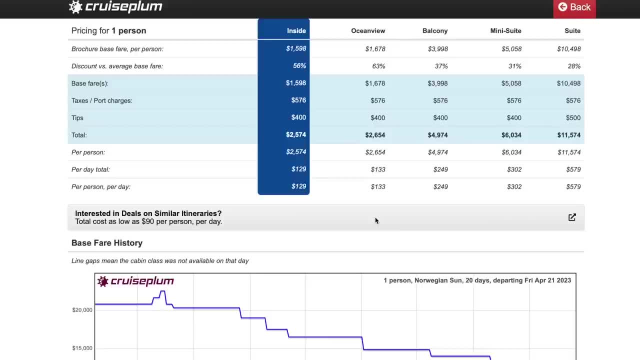 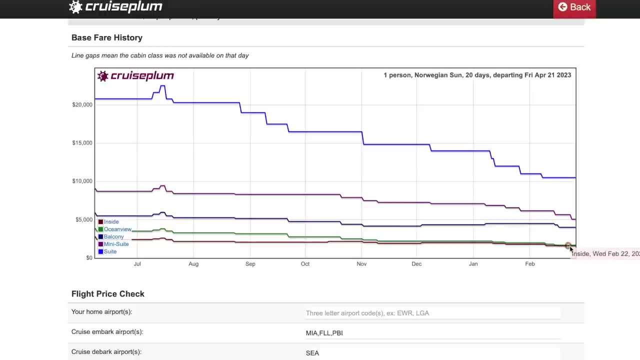 cool to have an ocean view and it might be worth it to pay an extra four bucks a day. you can also see the history of the cruise and where the prices went over time. you can see this one's steadily trending down. it's getting ready to happen, but 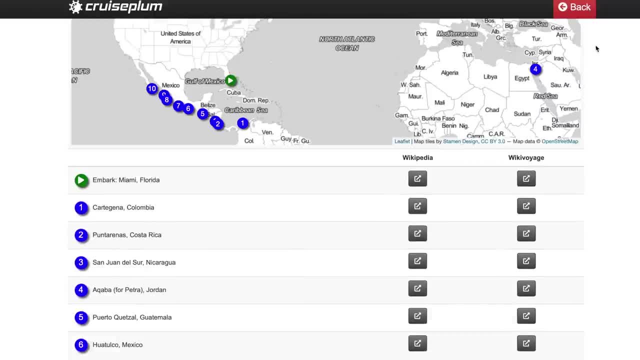 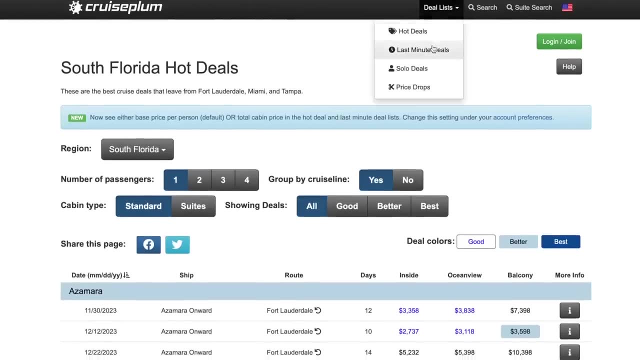 it's just got great data and then you can obviously see the different port visits and things like that. i don't want to go too much in the weeds there, we'll do that in a moment. but yeah, this is the hot deals tab. then you have the last minute deal tab. there's a much better way. 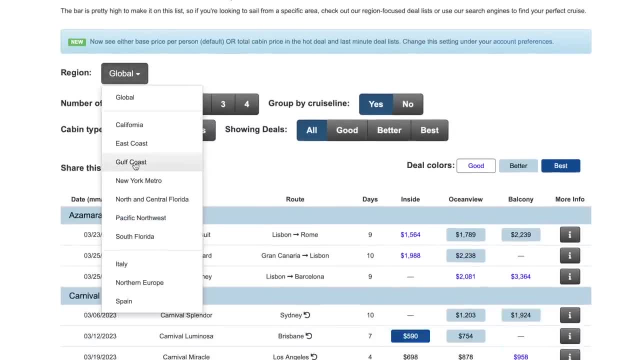 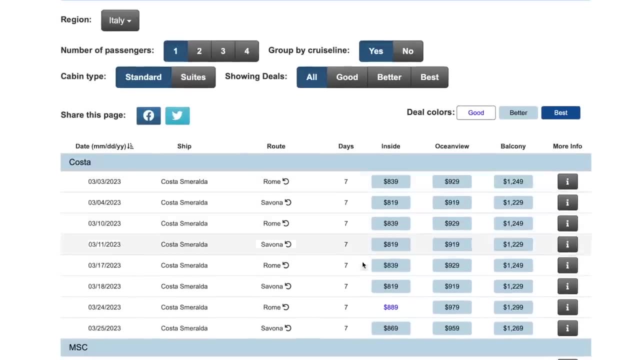 to find last minute deals, which i'll show you in a minute. but again, you can break it down. you can search the whole world or you can break it down and say i only want to see the hot deals. out of italy, you'll see a bunch of costa that are pretty affordable. out of italy, a bunch of msc that are 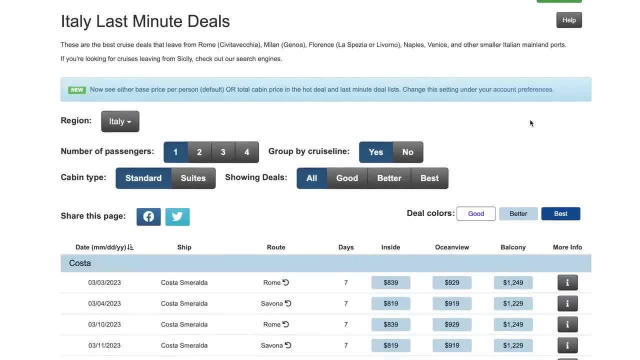 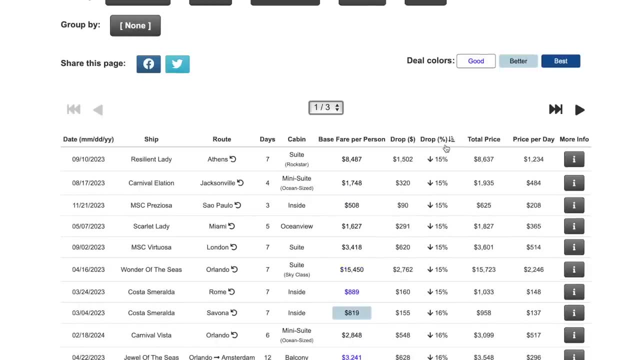 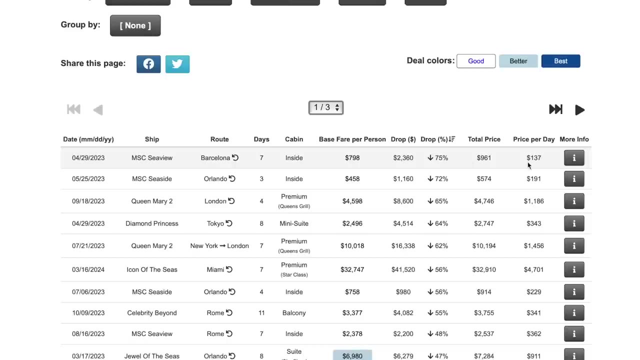 pretty affordable and same thing, you can click and get data on that specific cruise. and then i wanted to show you price drops. you'll see here you can sort it by price drop, which i love, and you can say: okay, this msc cruise, dropped 75 percent, might be a bargain: 137 dollars a day. 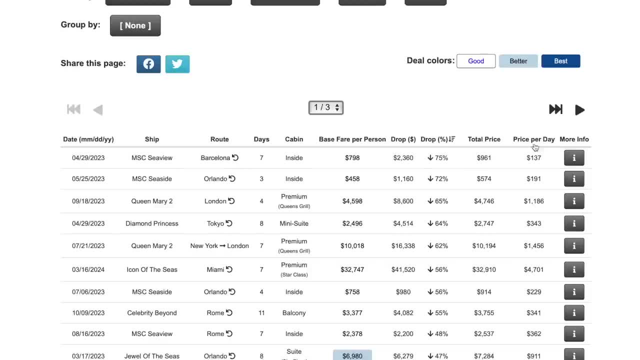 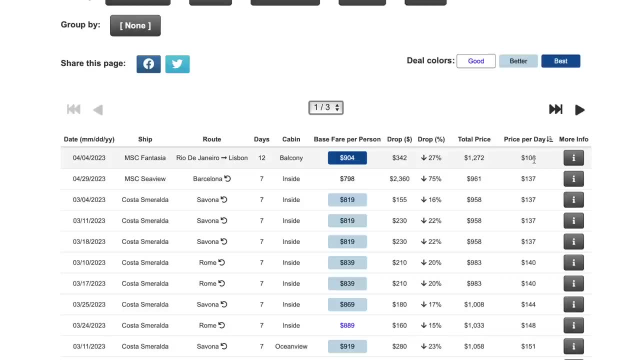 for an msc cruise. this is how i judge the price of a cruise. that's not really a good deal. let's sort by price per day and look, here's a cruise on the exact same or on a msc fantasia and it's 106 a day. obviously it's out of rio, but that's a good deal and you'll see. 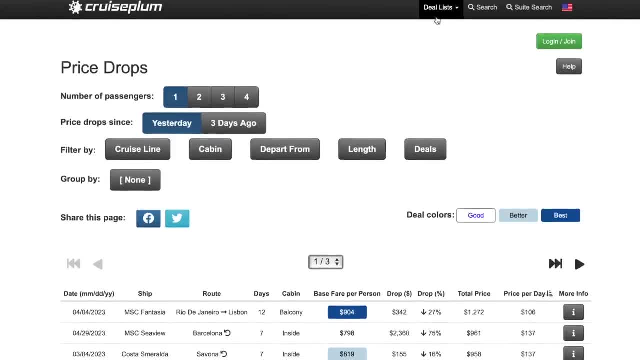 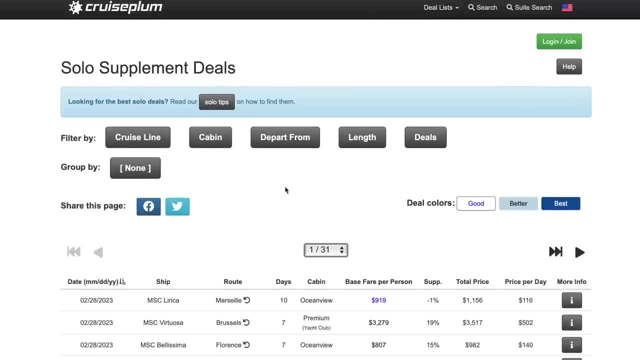 in a moment much cheaper cruises than that by cost per day. these drop down menus are kind of limited in the data they provide, so that's why i don't really go to them. but again, you can search by solo cruise and you can. if you are obsessed with supplement, you can search by supplement. oh my god. look seaside, 51 below supplement. wait 178 dollars for a day, an msc cruise inside cabin. that's not a good deal. that's not a good deal even though your supplement is 51 less than what a double occupancy couple would pay. it's again like i mentioned earlier. 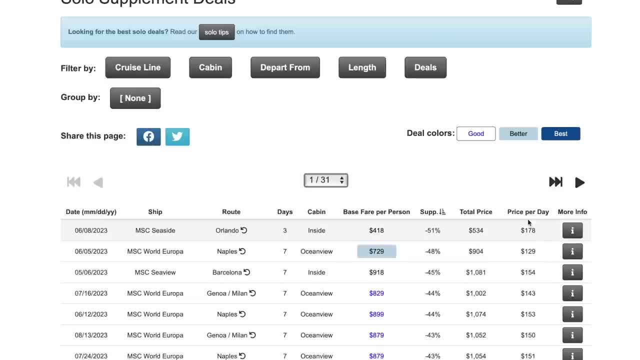 it's not a good indicator of a good deal. this is your indicator of a good deal and if you- uh, actually let me go back here- if you sort by price per day on here, you'll see these are a good deal right, this one's three percent supplement, you know. the other one was negative fifty percent. 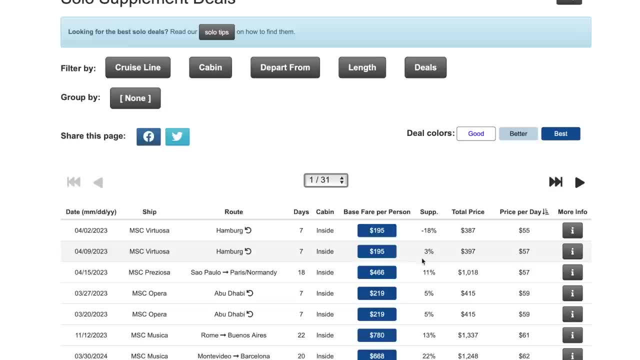 but it's only fifty seven dollars a day. so you can see why supplement cost or double occupancy, all that kind of stuff is not a good indicator of a good deal. you would think the negative 51 supplement would be a better deal than actually paying three percent supplement, but it's not. 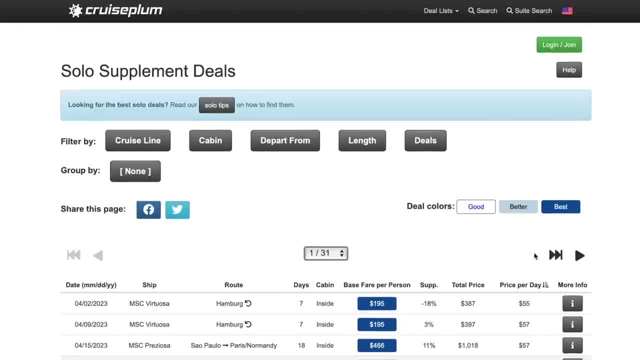 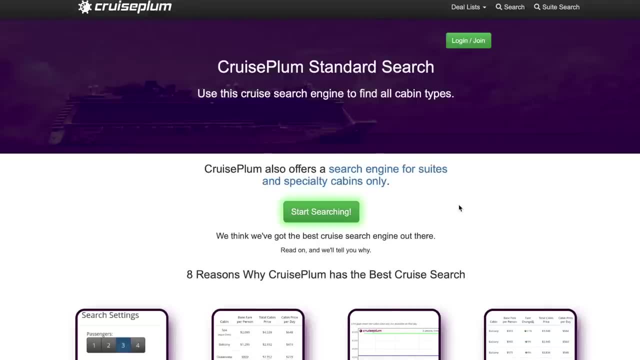 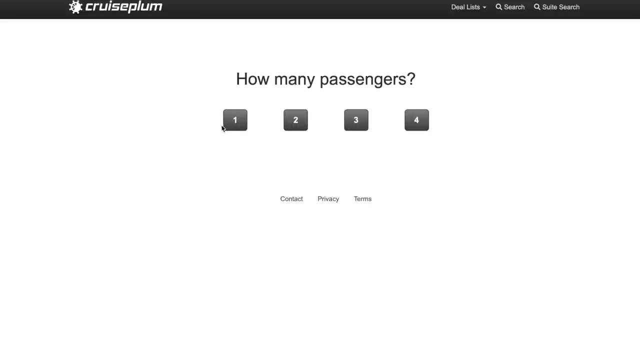 it's considerably cheaper here, right, but we'll we'll talk about that more later. so let's jump into the real search. uh, the the thing that makes this thing super powerful, in my opinion, because you can narrow it down to so many different things, which is great. so you click, start searching. you. 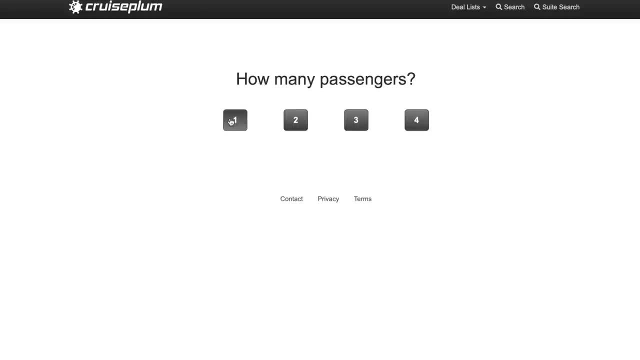 select the number of passengers. this will give you the price based on number of passengers, which is a great tool. it only has country of residence- us and canada. these guys are always updating this and adding more functionality, and so i assume in the future you'll see more nationalities. 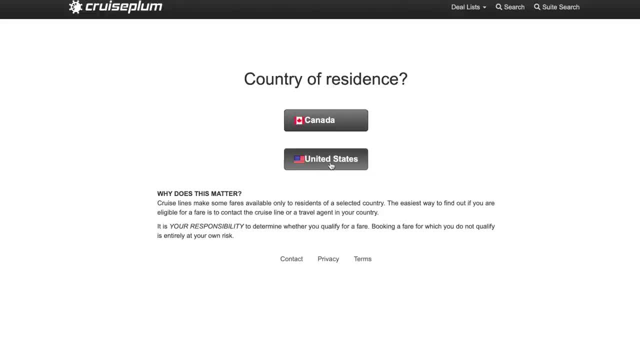 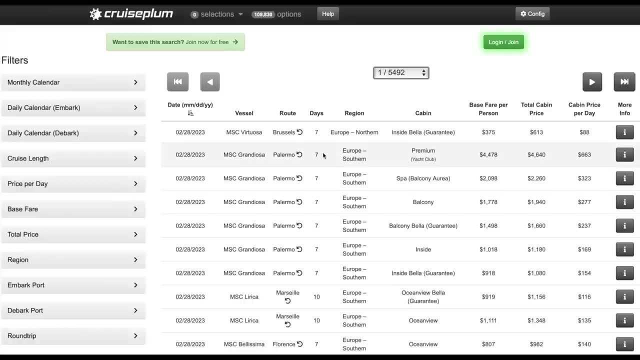 represented, but you can still search cruises out of anywhere in the world and hopefully, you know, in the country you're in maybe they'll, you know, honor the price that it's showing you. uh, i'm not 100 sure on that, but you, you can search out of anywhere in the world and i'll 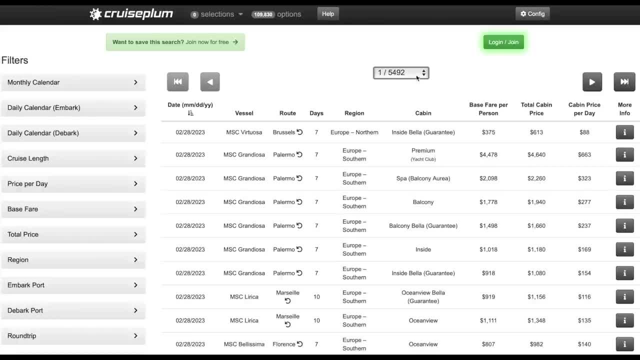 show you that in a moment. okay, so here we go. we got 5 000 search results, or 5 000 pages of search results, here and you can sort by a bunch of different things. right now it's sorted by date, so you can sort, you know, if you're- hey, i want to take a cruise tomorrow, you can look right. 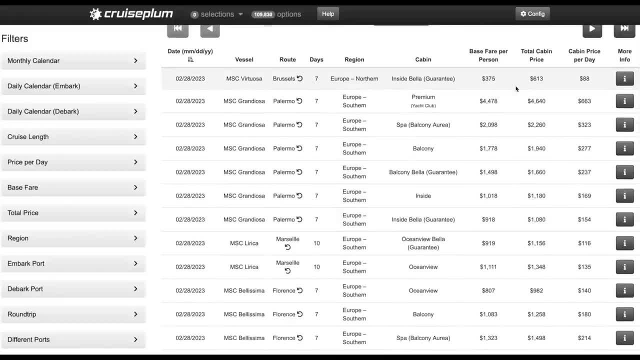 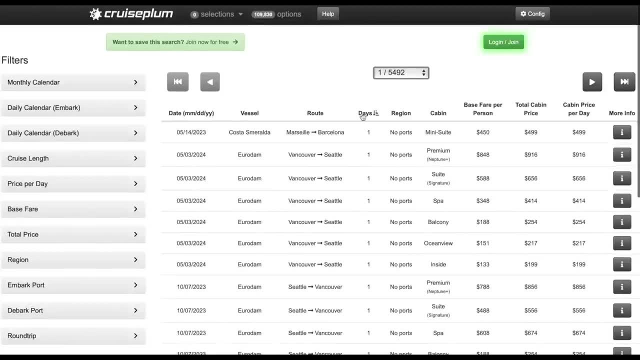 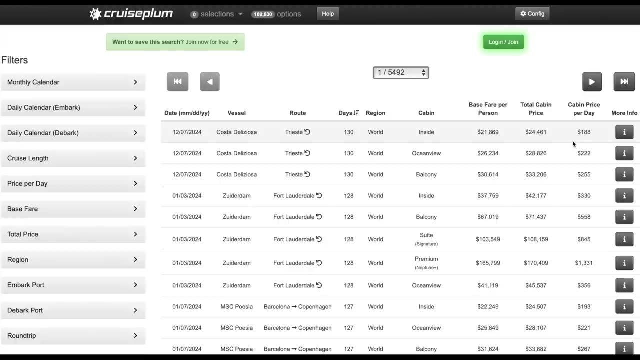 away at what's available. like you could hop on msc virtuoso right now for seven days for 88 bucks a night, so you can sort by that. you can sort by vessel route, number of days. like me, i'm always looking for really long cruises. look, here's 130 day world cruise on costa, 188 bucks a night. i don't. 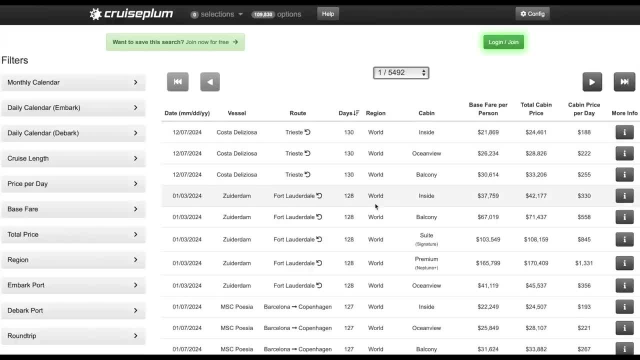 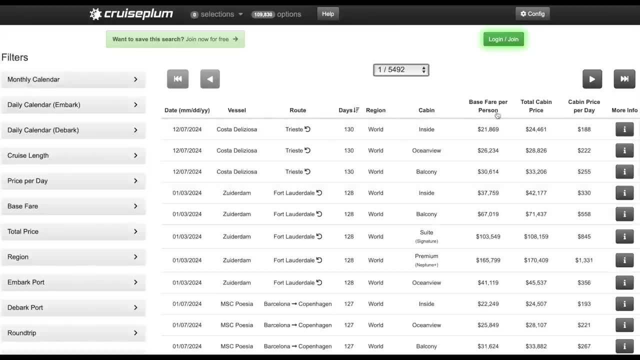 i wouldn't consider that a good deal. but you know you can do that. you can sort by number of days, which is great. you can sort by number of days, which is great. you can sort by cabin and you can limit all this stuff which i'll show you in a moment. and, of course, my favorite indicator actually. let's see what. the most expensive cabin is on here right now: wonder of the seas- 12 000 per day for a premium star class cabin. that's the most expensive one listed on here right now. the cheapest msc virtuoso out of hamburg: 55 bucks a day and you'll. 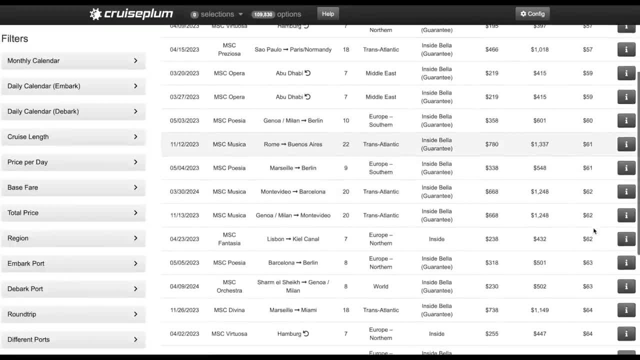 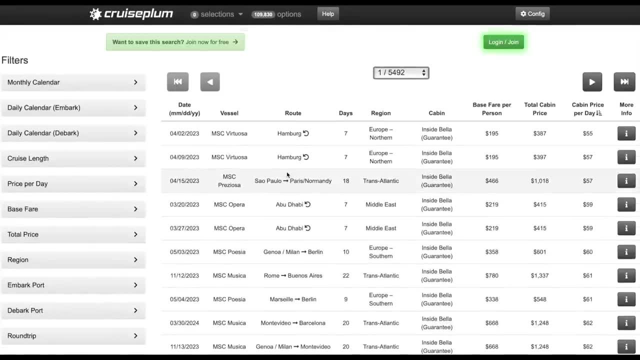 see a bunch of msc on here for most cost effective. it's just something you're going to see here and i like. ah, that's just clogging up my view. i don't want to see a bunch of msc cruises. i don't like msc. 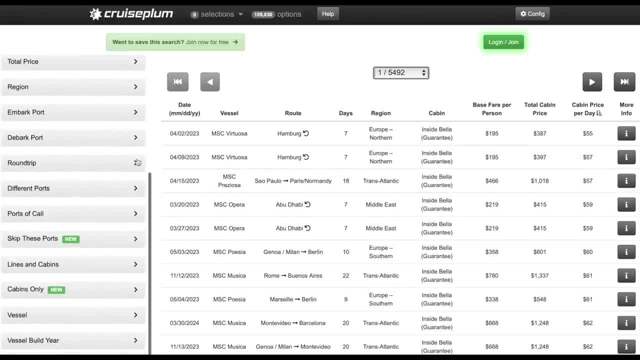 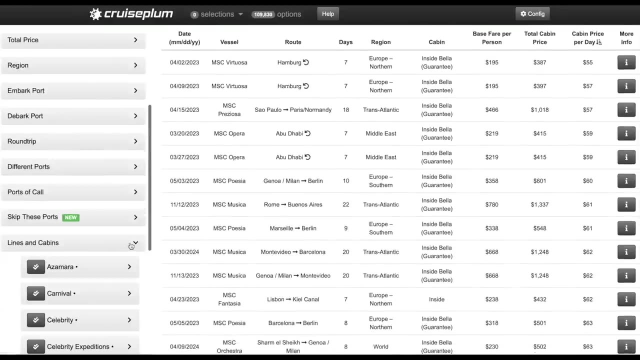 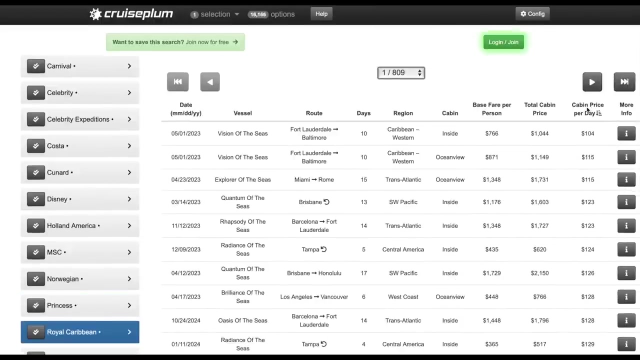 kevin, i like to cruise on royal. i'm loyal to royal. okay, well, you have all of these ways to narrow things down, so you can go here and say i just want to look at- uh, you know, royal caribbean. so you can go here, click on royal and now it's just going to show me the role i can look at cost. the cheapest rural cruise right now. vision of the sea is out of fort lauderdale. 10 day cruise- western caribbean- 104 a night for a royal caribbean cruise. that's freaking awesome, and i know what you're thinking: 10 days divided by 766, that's not, that's 76 a night. why is it say 104 a night? 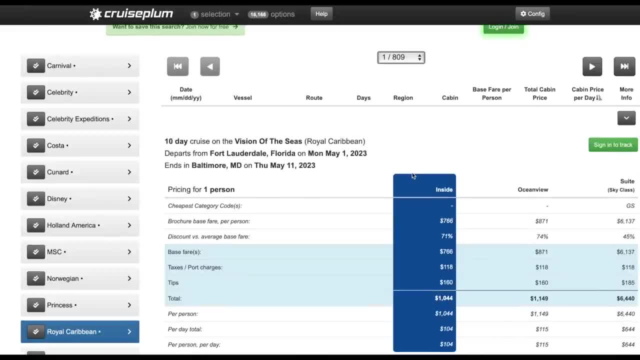 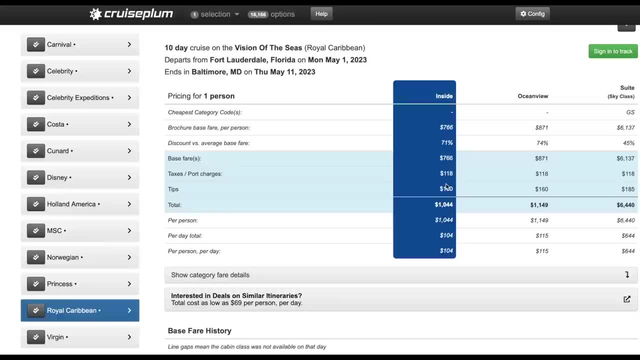 because that's the total price that includes everything you would have to pay for the cruise. that's what i love about this: it shows me the real cost of the cruise. it shows me base fare, taxes and port fees and the tips when it's called, you know, for big mission. these four, like this, are: really gorgeous. i'm mean, i don't know why people do say it depends on the speed. don't be just lockers. unless this one was on board, i'm just gonna tell you it was lost afterward. you know the ridiculously cheap cruise abc max-to-marine, aren't you? it's all it's amazing. and that the bottom line was thathet back then. it really 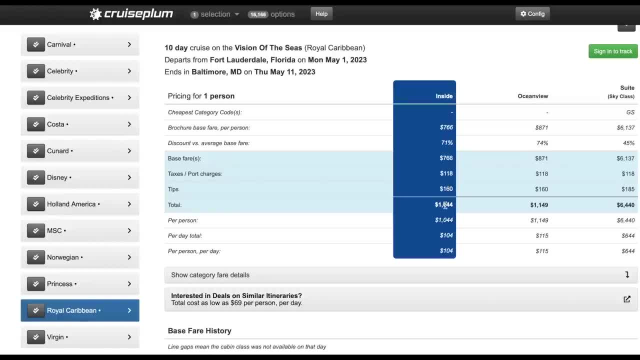 it's calculating the number in this main search engine and so i can see: all in, on this cruise i'm going to pay 104 a night. that's what i love about this: i'm not clicking on what seems to be a great deal and realizing port fees and and and tips. you know, push the price up, you know, double, i know. 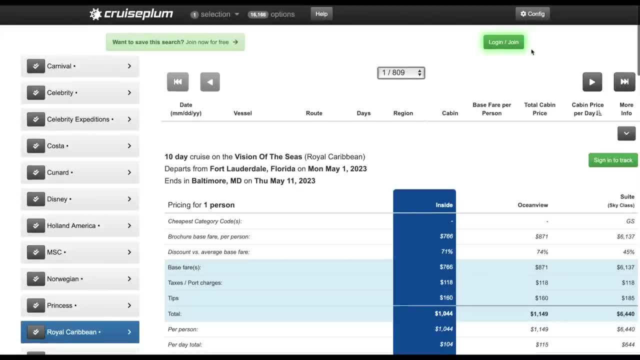 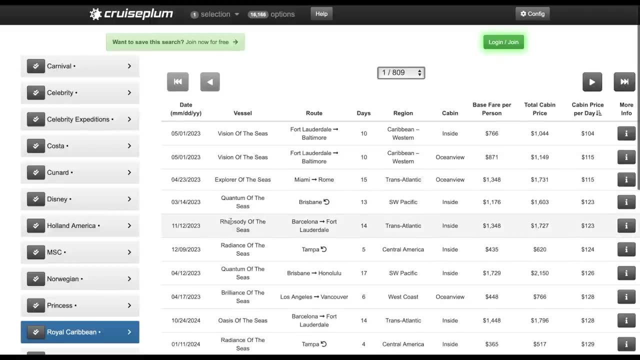 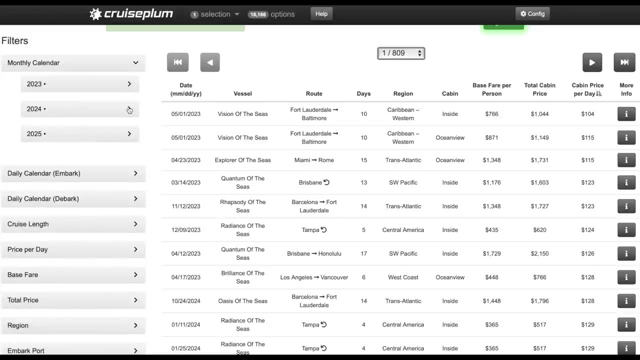 exactly what the cruise is going to cost me when i'm using this search engine, which is, you know, awesome. okay, so let's say you're like: well, you know, like this is all mixed up, i don't know what day i want to cruise. you can sort it by day. you can look by month, if you know you want to cruise. 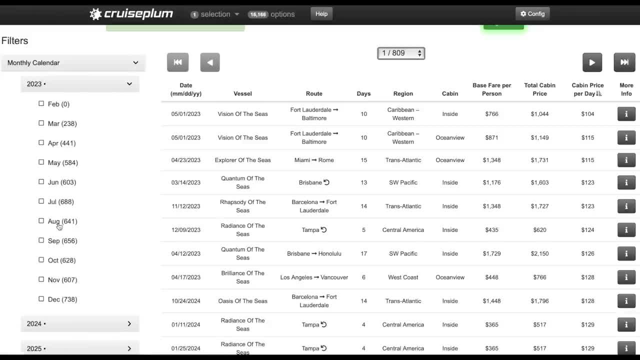 in june, if you know you want to cruise in, let's say, september of 2023, you can. you know, just look at september 2023. if you want specific days, like for me. a lot of times i'm jumping from cruise to cruise and you know i pull in on a lot of the like, the like four or five days. i'm just like you know. 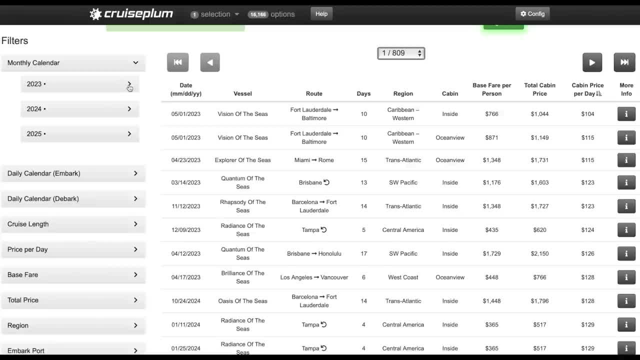 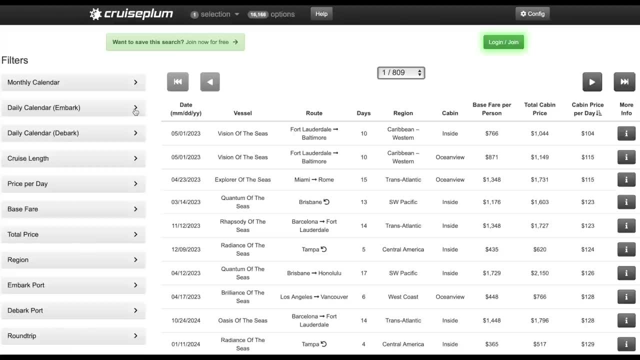 a saturday and i either want to jump on a cruise in that same port on the same day or i want to have a day in between and fly to a new port where there's a cruise. so we want to look at daily, right, so you can sort. that's what i meant. you can sort by the day you need to sail. so let's say, i'm 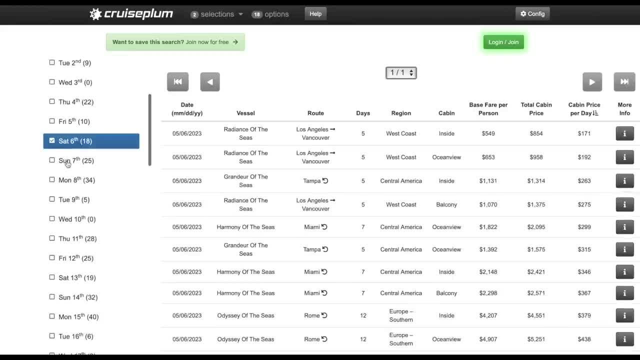 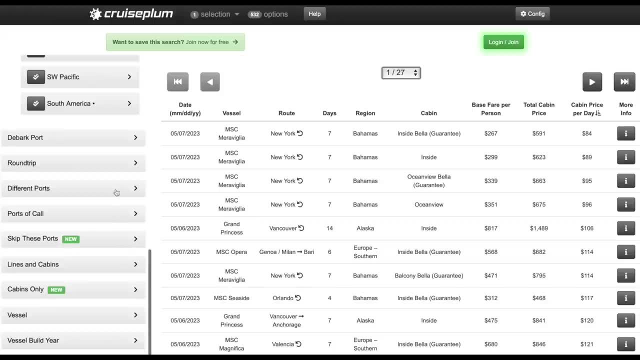 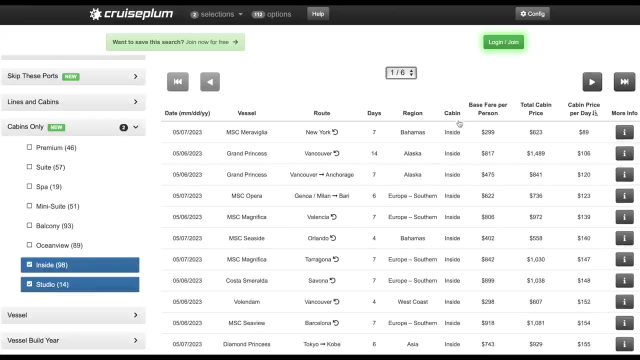 coming in on, you know, saturday, and i'm also going to select sunday, because if i have to fly to a new port, i can do that. if you only want to look at inside cabins, which i always do, you can just select studios and inside cabins. so now, all i'm going to see right now is inside cabins and studios. 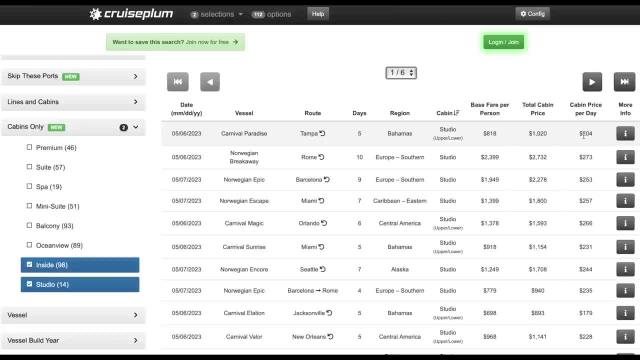 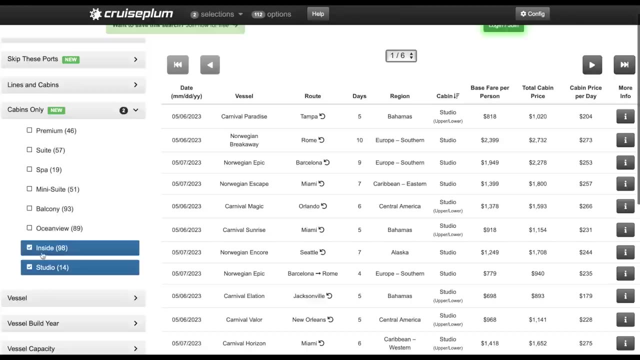 let's say i want to see the studios. okay, carnival paradise, they have a studio. look at how expensive per day that studio is. studios are not a good deal, all these studios. look at how expensive they are. here's one: 179. that's like the cheapest one. but yeah, you can sort by the cabin type, so you can. 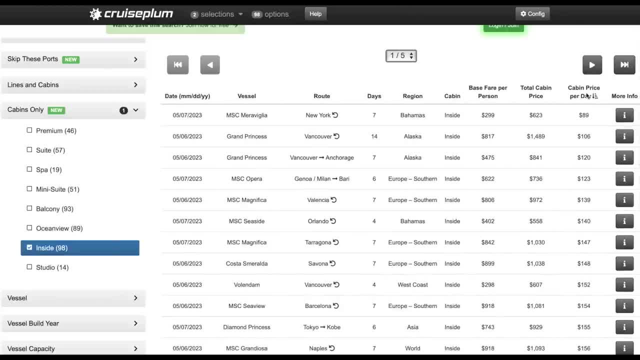 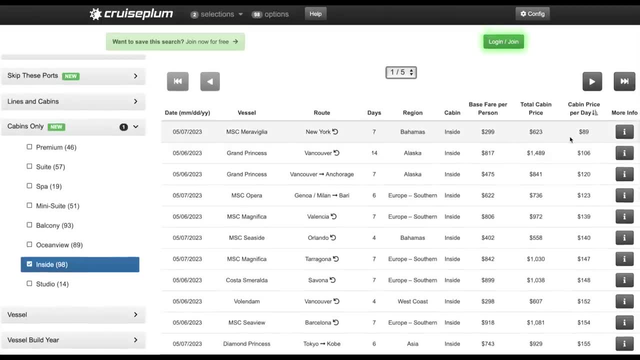 get rid of a lot of cabin junk, lot of the muck that you see in, you know, when you're searching. here's MSC Maravilia. we were just talking about those dates I put on there, so this is probably the one I would do. I would just. 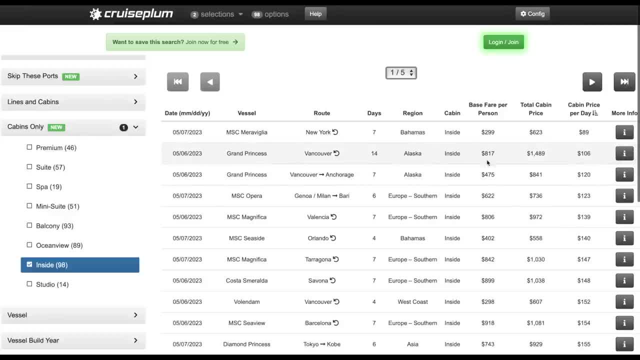 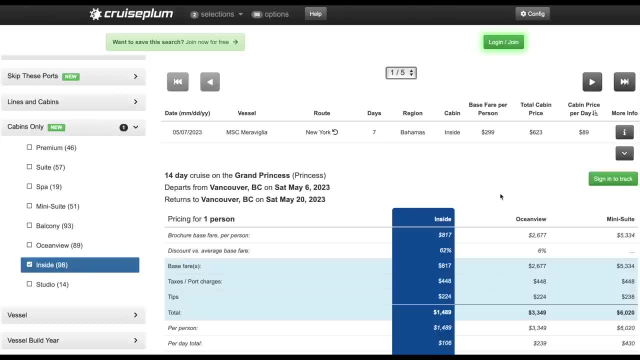 fly up to New York, or maybe I'd fly. actually, you know what I would probably do in this scenario: I would fly to Vancouver. I would fly to Vancouver and jump on this Grand Princess cruise. like $106 a night for an Alaskan cruise, like that's a great number and it's on Princess, which I love. 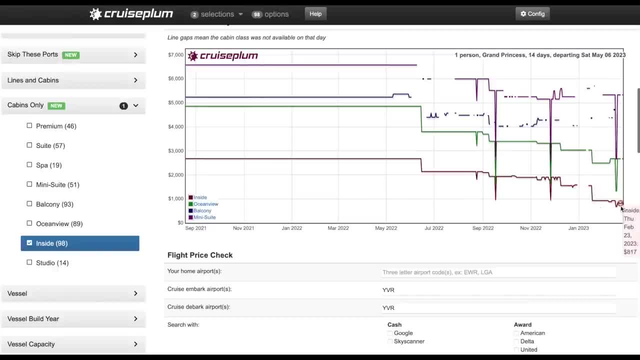 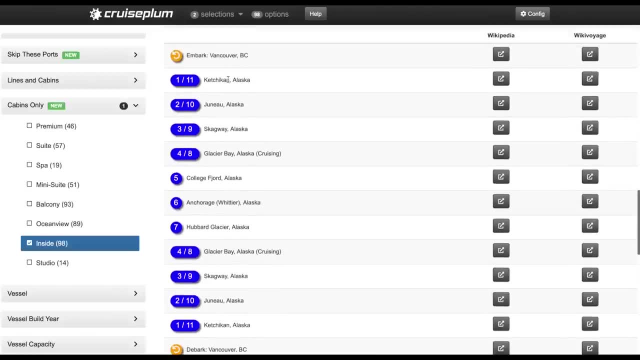 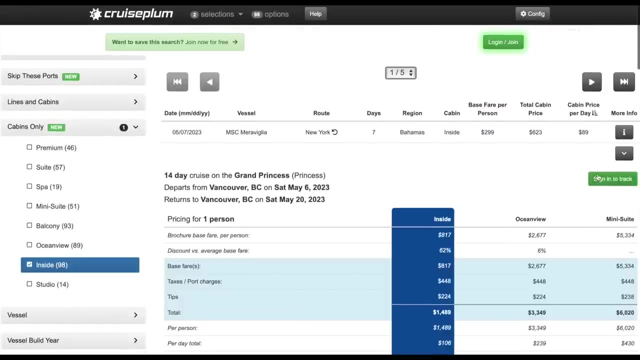 you can see here. you can go into finer detail here on price, but look at that itinerary. that's awesome. Vancouver to catch a can- that's awesome itinerary. I would definitely book this cruise if those were the dates I was working with. I just go ahead and fly to to Vancouver. 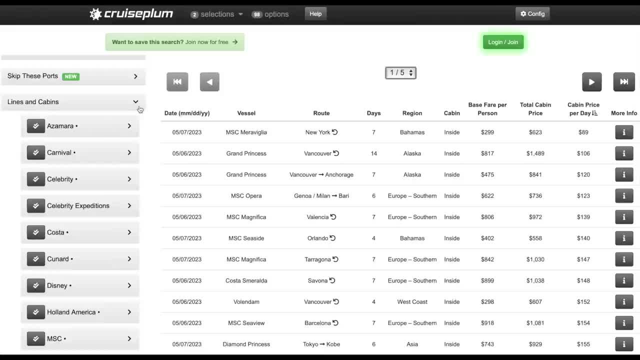 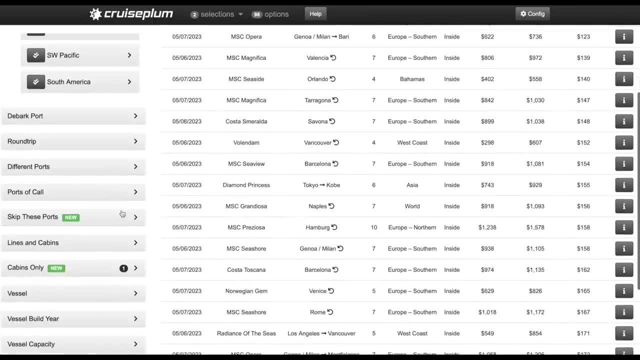 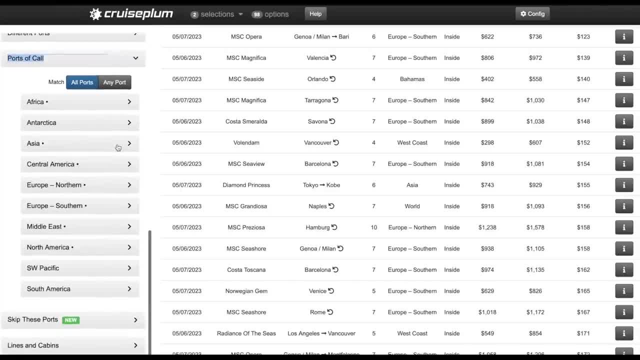 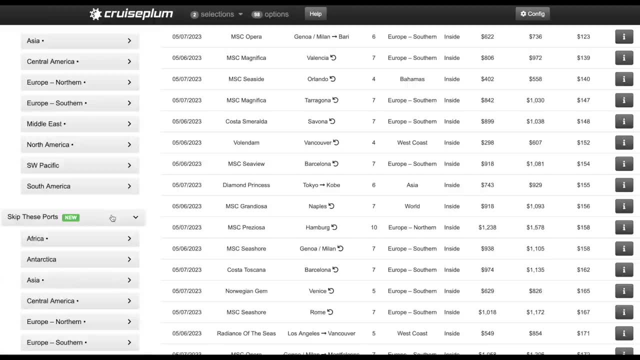 Venice and a port of call. you can search by. you know cruises that go to ports that you want to go to. or hey, I want to skip these ports. I don't want any cruises that go to Nassau, Bahamas, because a lot of people don't like Nassau. you can search by that. I mean, it's just so much you can do you. 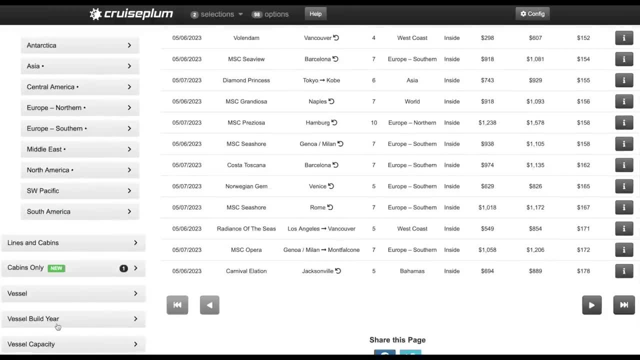 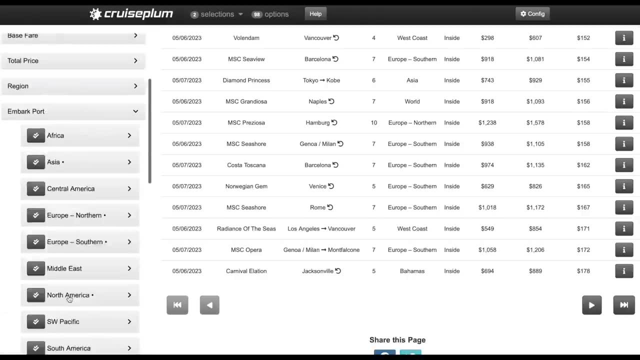 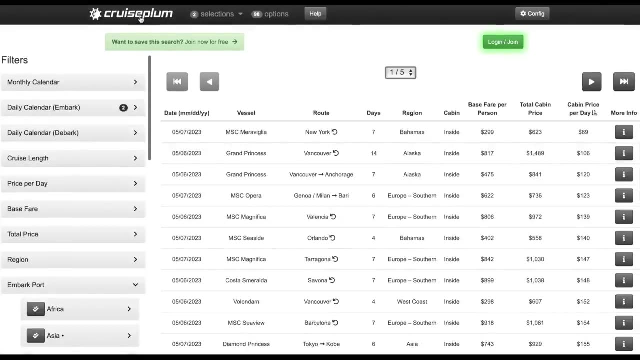 can go by vessel capacity, vessel year. I don't want to sail on any old ships, you can do that. I don't want to sail on any new ships. you know it like the functionality of this website. you, it's just amazing. so that's why I like it so much. okay, now let's talk about what all of 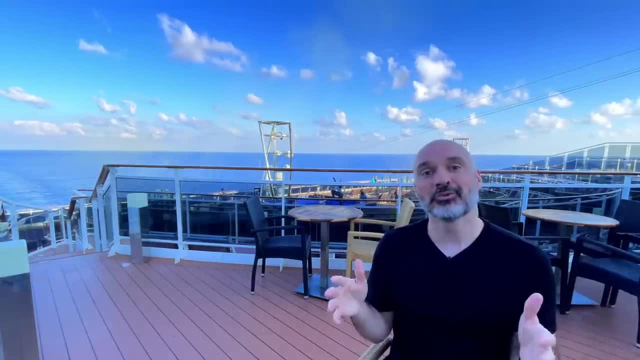 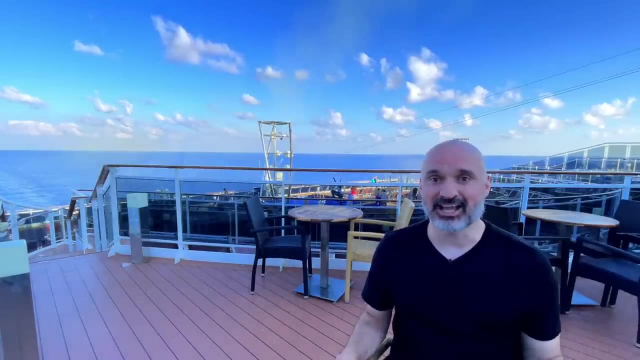 you've been waiting for how to save some money on cruises, some tools and techniques to use. I use a couple different techniques and websites and things like that. so the first one, my friend Andrea, who I met on Sky Princess. she turned me on to this website. it's called Sky Princess. 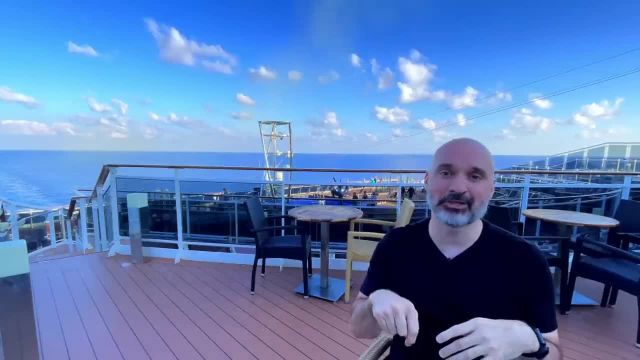 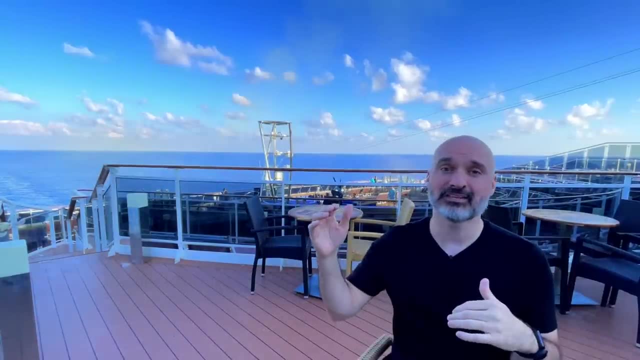 it's called Rakuten or something like that. I'll put it up here. there's a link down below and if you sign up, I think they give you thirty thirty dollars right away. this is a cash back website, so you don't get any money off your cruise, but once you book your cruise and pay for it, you get. 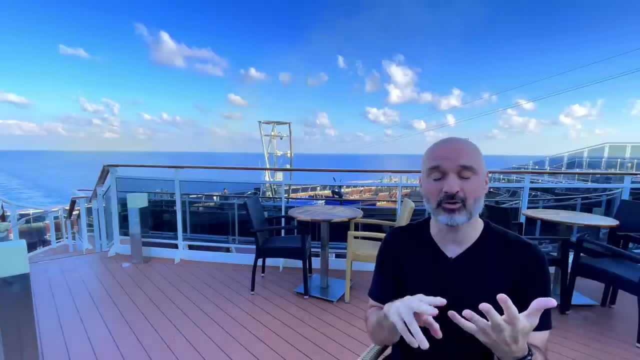 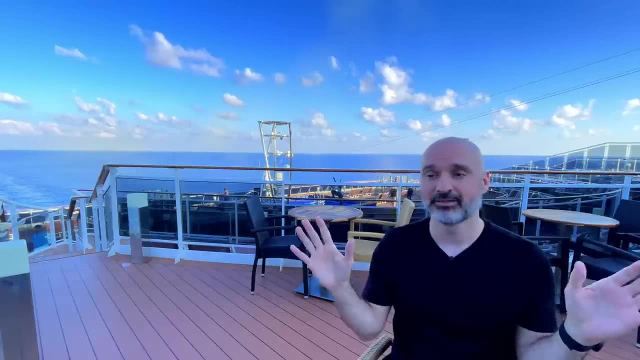 money back from them, and they do it one or two ways. they'll pay you via PayPal or they'll send you a check. I've done it before. it worked flawlessly. they sent me the money through PayPal. it's completely legit. a lot of people use it for a bunch of other things, like you can buy Nikes and things. but they do have cruises on there and the amount you get back per cruise rotates. right now you can get 1.5% back on Princess, you can get 2% back on celebrity but about two weeks ago it was 4% back on celebrity cruises. they have celestial cruises and I'm sure it rotates and the percentages 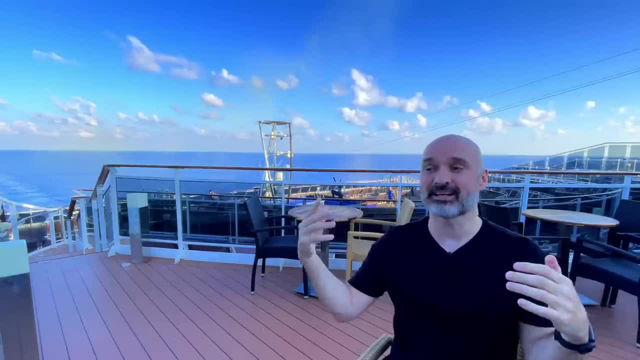 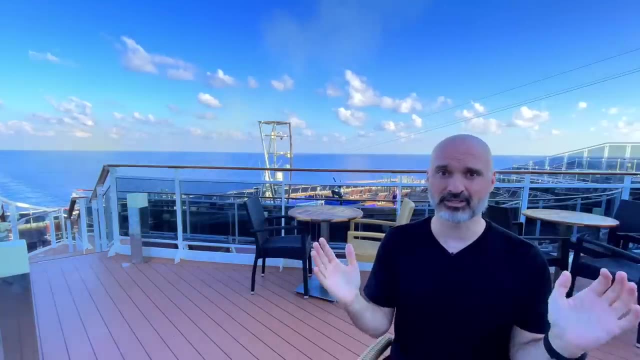 change. but it's pretty simple to use. you just make an account and I think if you use my link below they'll give you 30 bucks or something like that and you can refer friends like that too. I don't work for them or anything like that, they just have a referral program. 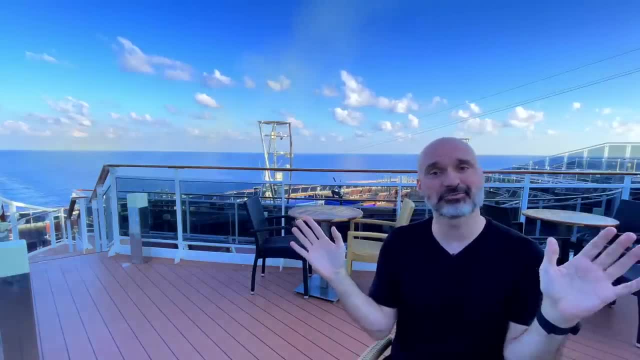 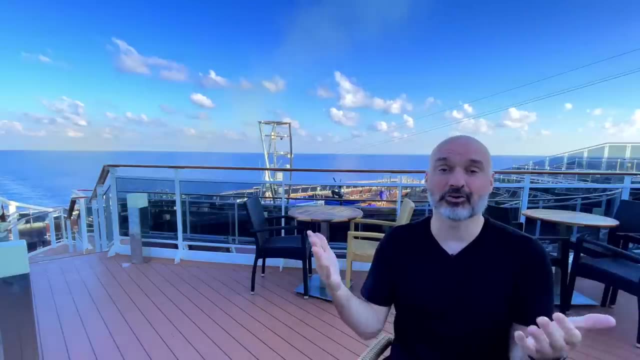 down there. you can use it if you want. you can use somebody else's referral if you have someone that uses that website, whatever, I don't care. it's just a great way to instantly get some money back on cruises that you book. if the cruise that you want to book you know they offer a discount another way. 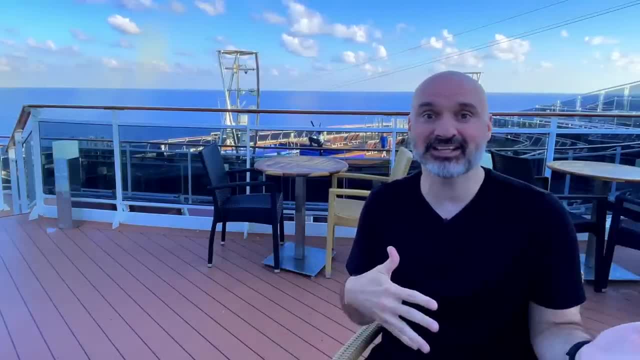 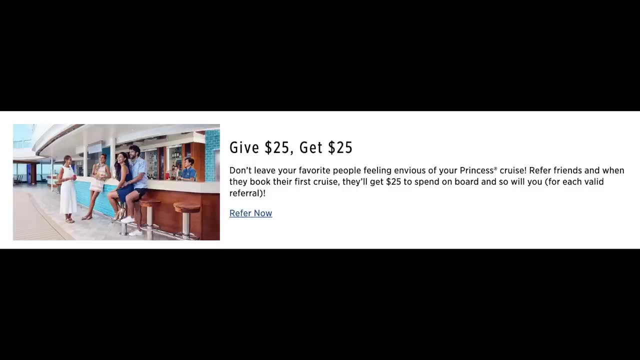 I save some money is through friend referrals with the different cruise lines, like: if you look down below, you'll see I have a referral for Princess. anybody can do this. I don't work for Princess, I don't have any kind of contractual relationship with them, but if you use the link down below, I 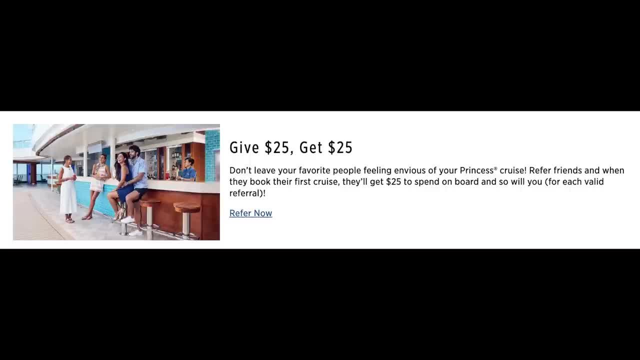 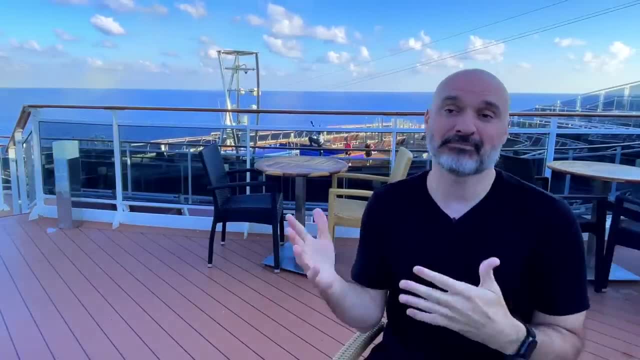 get $25 off your cruise and they give me $25 off my next cruise. so kind of cool. I think all the cruise lines have some kind of refer program. so find some of your friends that cruise and say, hey, do you have a referral link? they might not even know they have one, but anybody can get one if you. 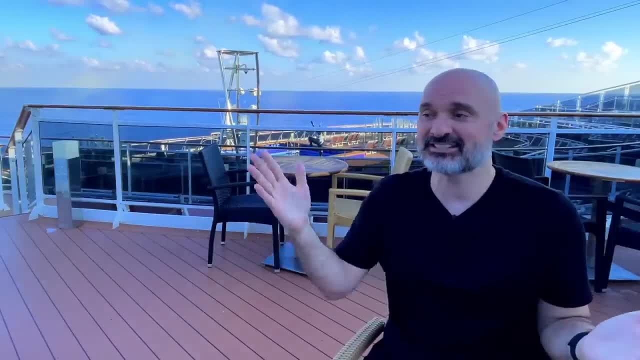 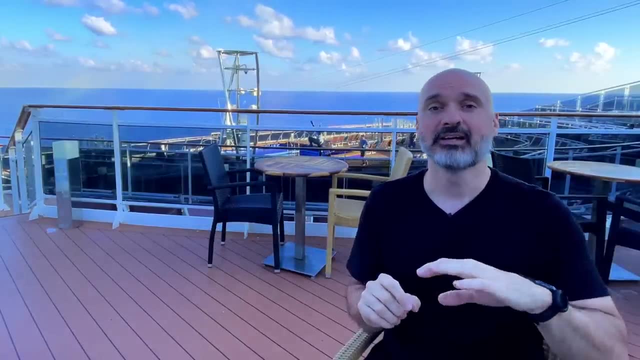 want to use my Princess- one down below you can. if you got a friend that Cruises Princess and you want to use theirs, just tell them to go get their referral link and they'll just get 25 bucks off their next cruise. so that's another great way to get some money off your cruise. another one is a. 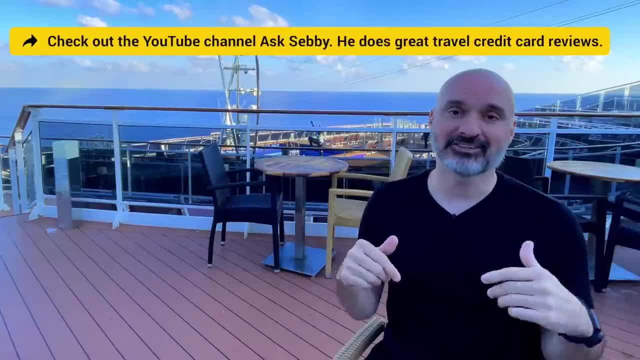 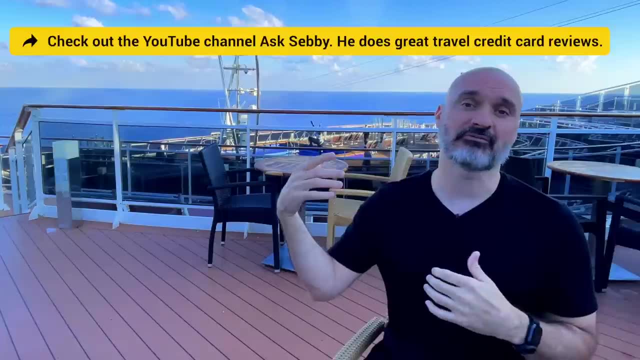 credit card point system. me I use Chase Sapphire Reserve. again, there's a link below. but figure out what credit card system works for you, where you get points that you can redeem for Cruises. you can redeem for other different kinds of travel. I use most of mine for flights and hotels in between Cruises. I haven't.